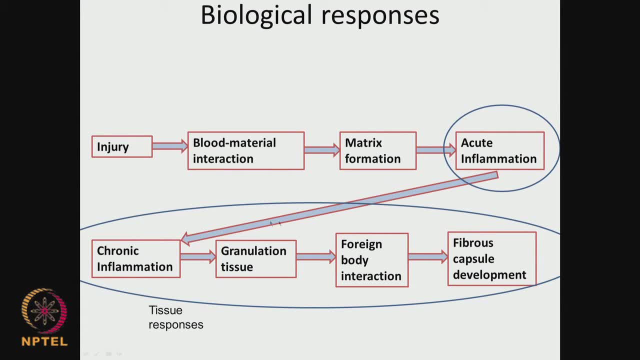 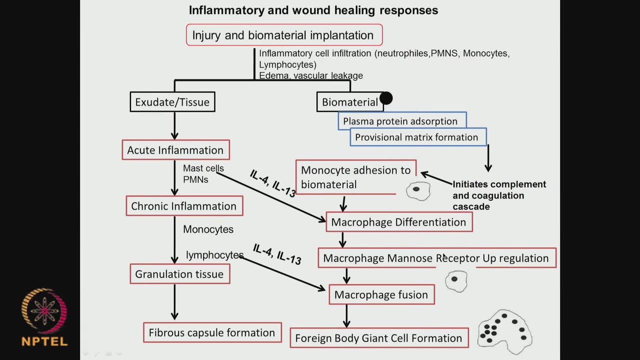 response: acute inflammation, the chronic inflammation, then the tissue formation, foreign body interactions and fibrous Encapsulation of the material and so on. actually, So lot of tissue response starts happening here, So we will look at it slightly in more detail. So when there is an inflammation, there are 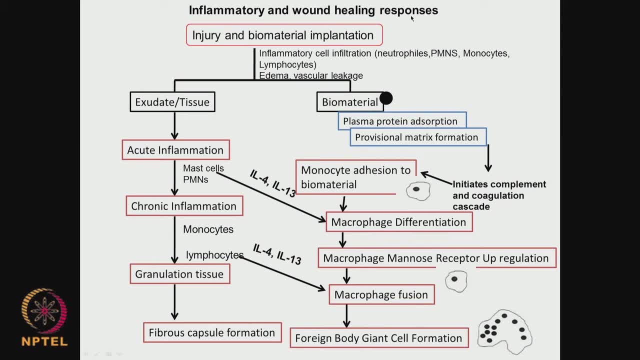 lot of wound healing response because when the surgeon tries to open the host body and then place a biomaterial, obviously it is like a wound. So the wound healing processes start taking place Because the surgeon tries to open the host body and then place a biomaterial. 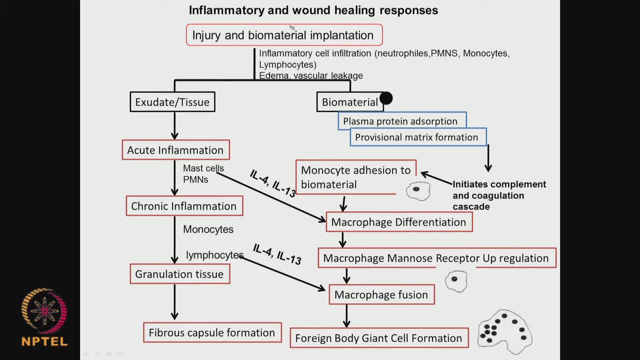 obviously it is like a wound, So the wound healing processes start taking place, because the surgeon has created an injury because of the biomaterial implantation, So there is going to be inflammatory cell infiltration. So lot of cells like neutrophils. 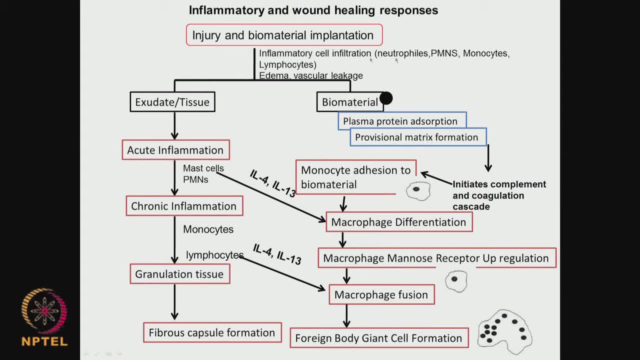 PMNase monocytes, lymphocytes, start going towards it, Then there is going to be edema, vascular leakage, So all these start happening actually. So the biomaterial is placed inside, So there is plasma protein adsorption. Then you have provisional matrix formation monocyte. 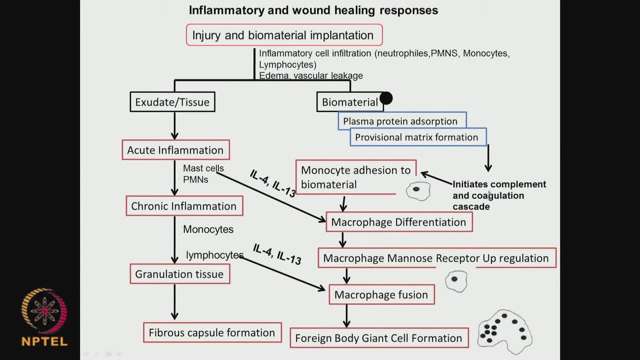 addition to the biomaterial, which here, you have the complement and coagulation which we talked in detail. Then we have the macrophage differentiation Macrophage plays a very important role in forming lot of foreign body giant cells and trying to engulf or encapsulate. 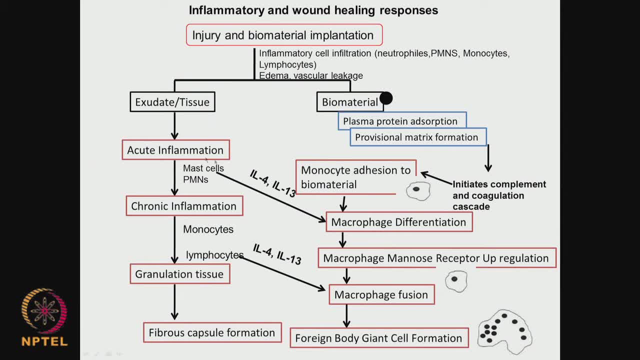 the biomaterial. So they are all interrelated. as you can see here. We have the acute inflammation, chronic inflammation, Then the tissues are formed here and your biomaterial gets completely fibrous: capsule formation. So both the things happen simultaneously when you have the inflammation healing process. 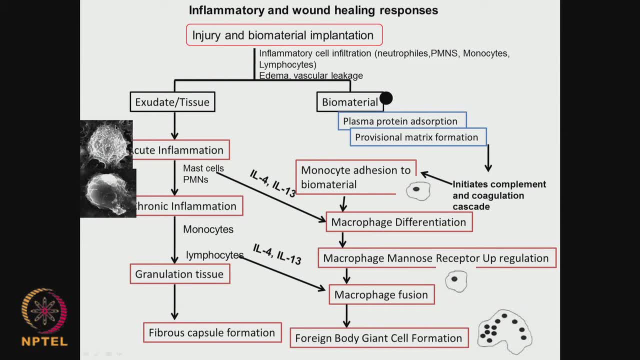 Now, these are some of the inflammatory cells, as you can see in this picture here, and these are granulation tissues. As you can see, these tissues are formed around the biomaterial and they try to completely encapsulate your fibers. As you can see, these are some of those monocytes which are formed near the site of inflammation. 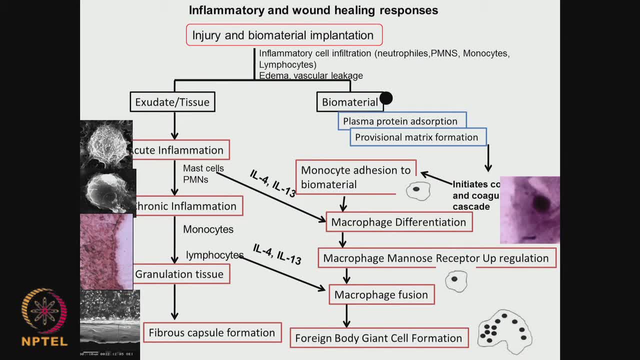 or near the site of where the biomaterial is placed. So these are part of the inflammation and wound healing process. So a lot of different types of cells are formed here. Then, finally, in the biomaterial is inert, It can completely get encapsulated. 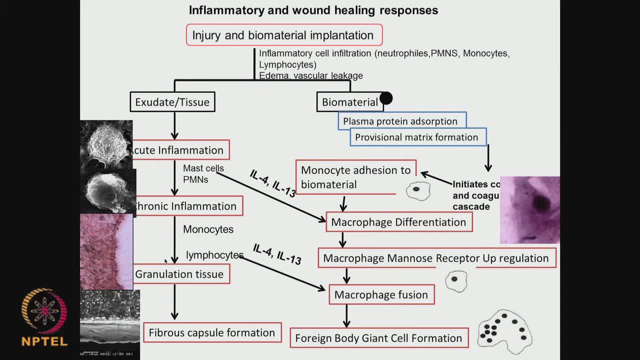 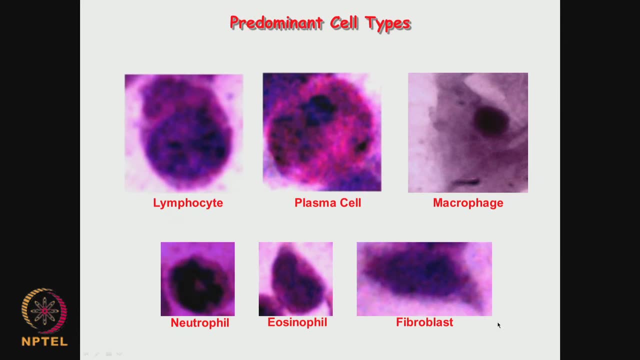 Of course, as I said, if the biomaterial is toxic or the exudant are toxic, then you could have cell death happening there. These are some again pictures of foreign body gene cell formation. As you can see here, this is called a foreign body gene formation. 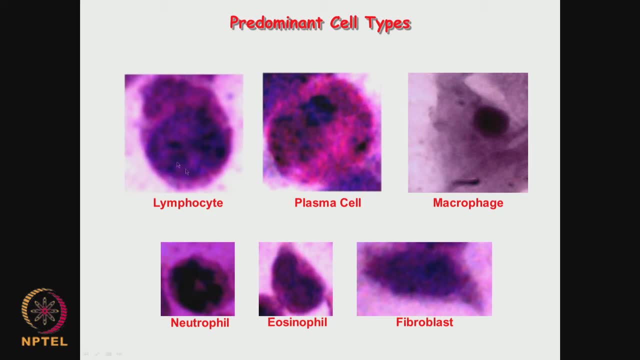 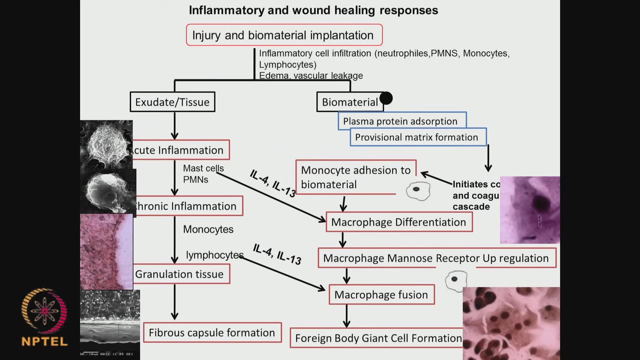 So different types of cells are formed. I showed this picture long time back: lymphocytes, plasma cells, macrophages, fibroblasts, neutrophils, xenophils- So all these are formed here in this particular step here. 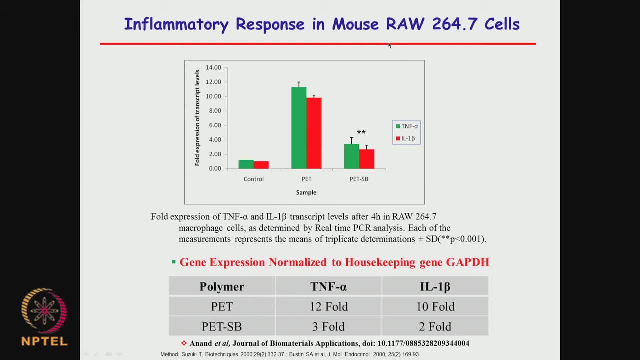 So look at this, there is an experiment. So when we use the mouse raw 264.7 cells, what happens when it is in contact with the biomaterial, like polyester? then this is a polyester, this is a modified polyester. So what are the inflammatory response? 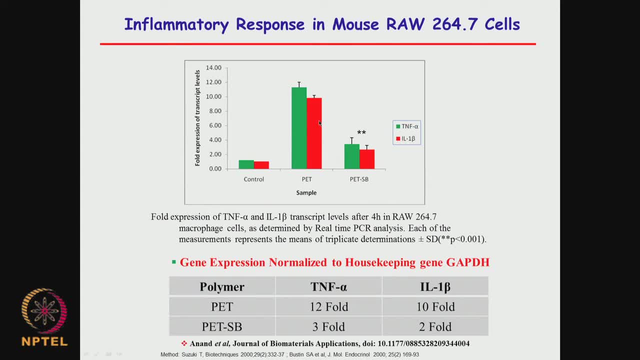 When the mouse cells are in contact with these polyester. this figure tells you the expressions of 2 important transcriptions which are involved in inflammation. One is called the TNF alpha, the other one is called IL-1 beta. These 2 are markers which tells you if there is an inflammation. 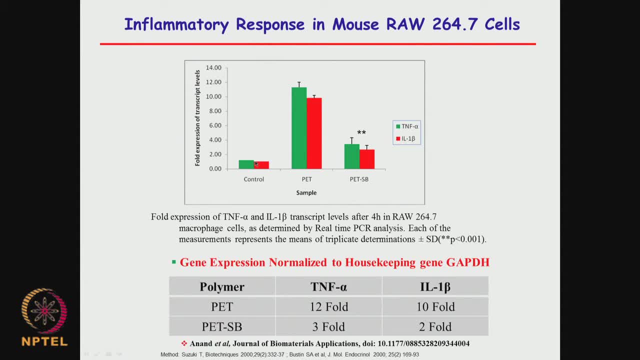 As you can see in the control, they are very, very low Amount of the level of TNF alpha as well as IL-1 beta. But as soon as they come in contact with the biomaterial made up of polyester- here so you can see- both of them have gone up tremendously, by almost 12 fold. 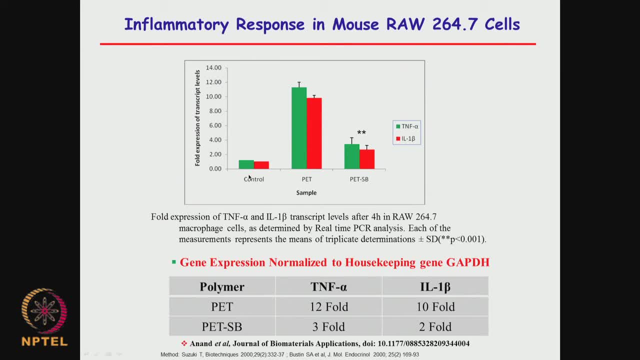 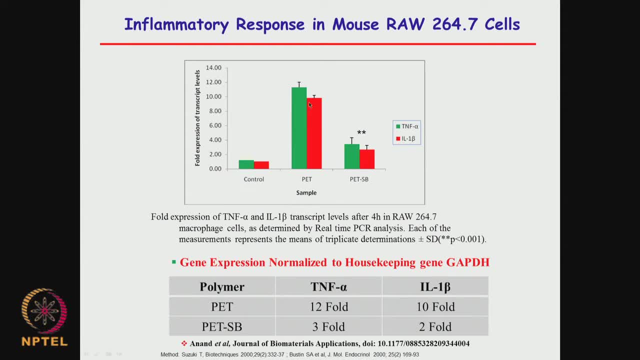 Polymers are not in contact with the biomaterials, So you are able to bring it down from almost 12 fold to 4 fold, So a 3 fold big reduction in the inflammatory response which you have achieved by modifying the surface. 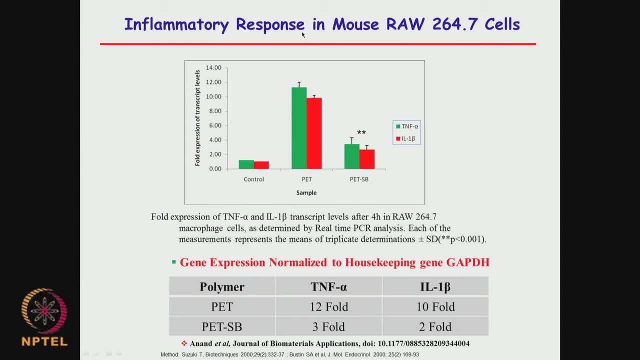 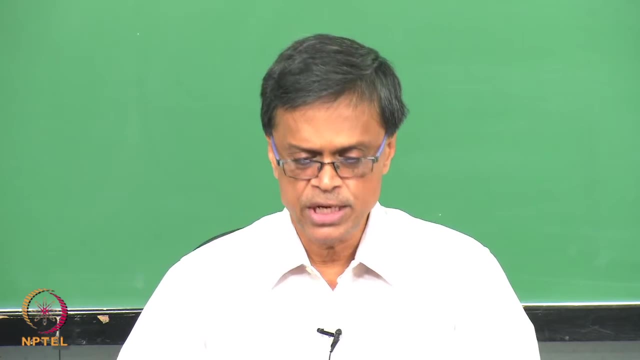 Because surface modification helps you to reduce the inflammatory response of the biomaterial to this particular cell line. So these type of experiments have to be done in your lab before you take the biomaterials further for animal studies. So these are called in vitro cell line based studies. 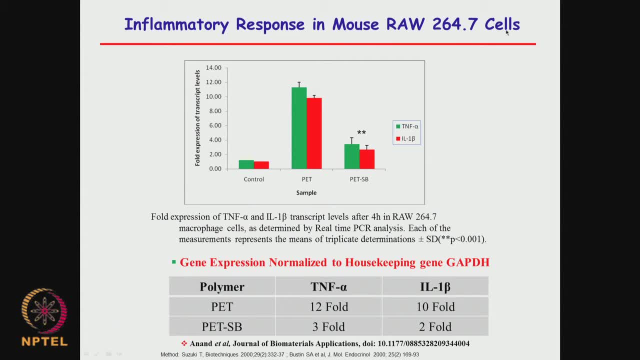 So we are using this particular cell line. You can test other muscle cell lines and so on And, as you can see, as soon as they come in contact with the polyester there is a big increase in the inflammatory markers. So most of the in vitro studies with cell lines. 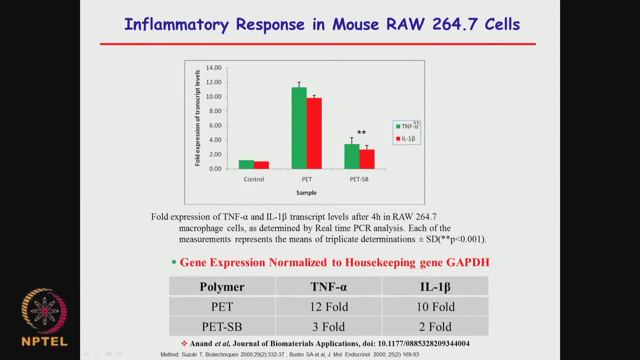 They are focused towards these 2 particular inflammatory markers. One is called the TNF alpha and the other one is called the IL-1 beta. So they look at the transcription levels of these 2 markers and then you will be able to tell whether the biomaterial is creating an inflammatory response. 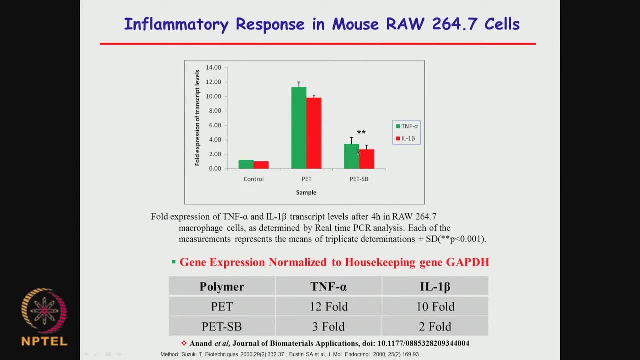 So we do some surface modification to this biomaterial and, as you can see, they come down dramatically, But still it is higher than the control, But it has come down dramatically. So how do you do these experiments? There is something called real-time PCR, polymerized chain reaction. 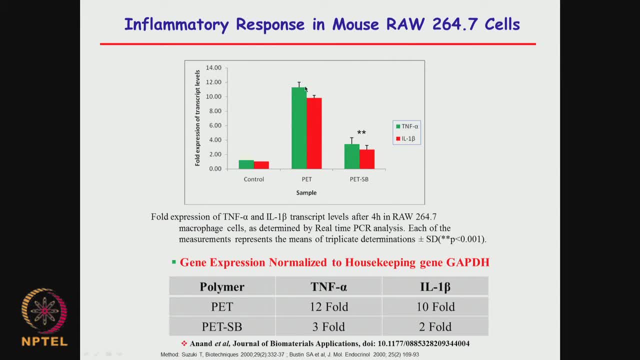 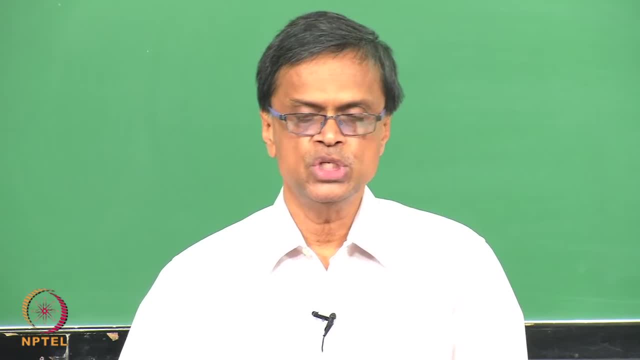 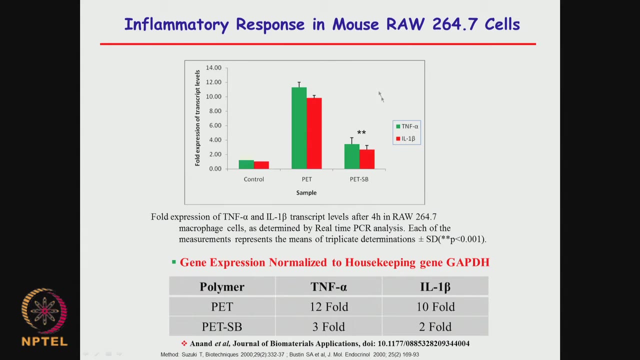 This is an instrument which can tell you what happens to various genes. So we can focus on a particular gene and then tell whether those gene levels are up when they are in contact with the material and so on. So it tells you the mechanism. This is called a mechanistic study. 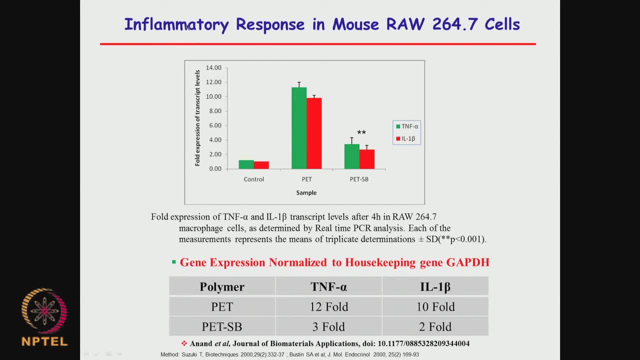 So we are able to tell there is an inflammatory response because these particular 2 genes, mainly TNF alpha and IL-1 beta, have gone up by almost from 1 fold to 12 times increase, And this one is 10 times increase. But when you do a surface modification you are able to bring it down to only 3 times. 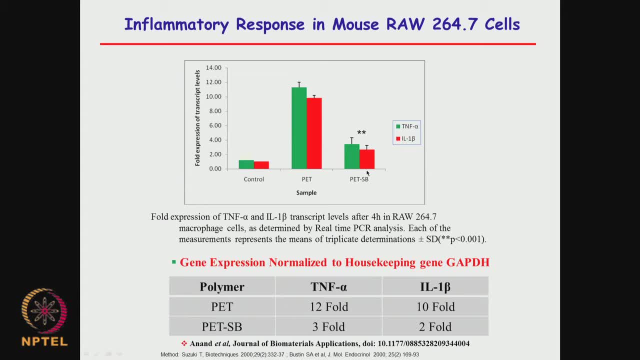 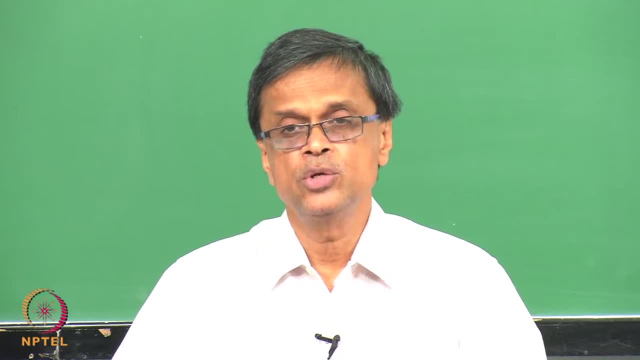 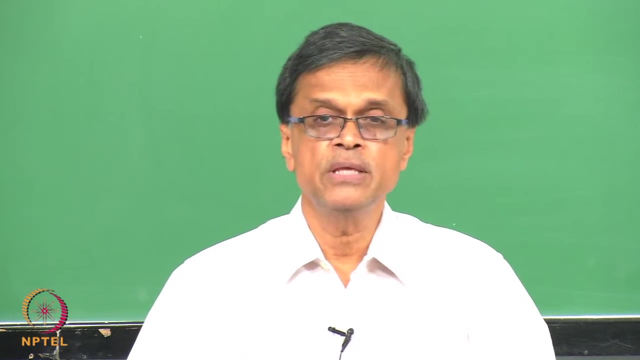 increase in TNF and 2 times increase in IL-1 beta. So do you understand? Yes, So this type of experimental studies are very essential to understand the inflammatory responses these materials create, And then we can modify the surface of the material so that the inflammatory response 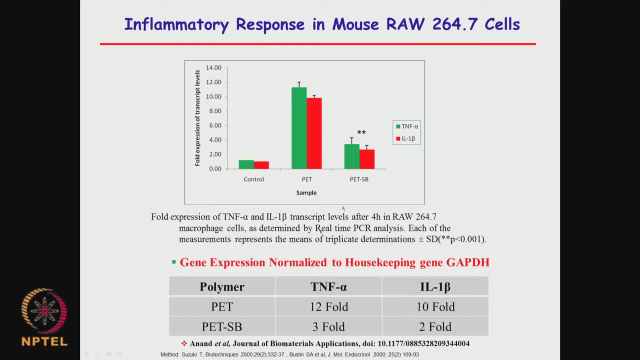 is dramatically reduced. So we may be able to reduce it still further by another type of modification. We will not go to too much into that as of now on surface modifications. but surface modification of biomaterial is a very important topic, veux topic. you can do it through different approaches: plasma bombarding, UV radiation, immobilizing. 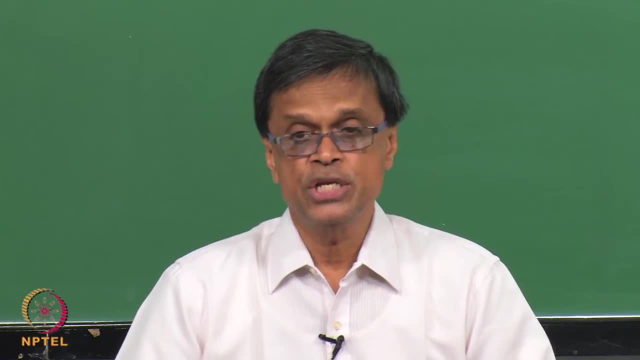 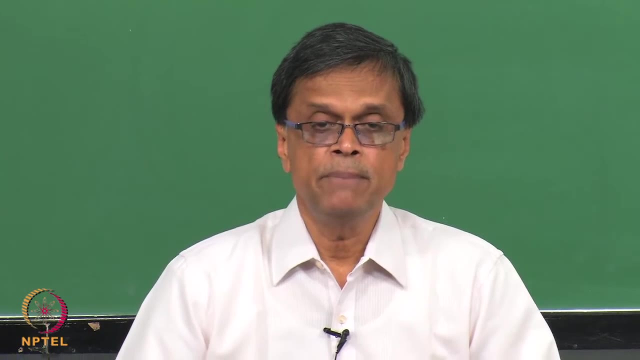 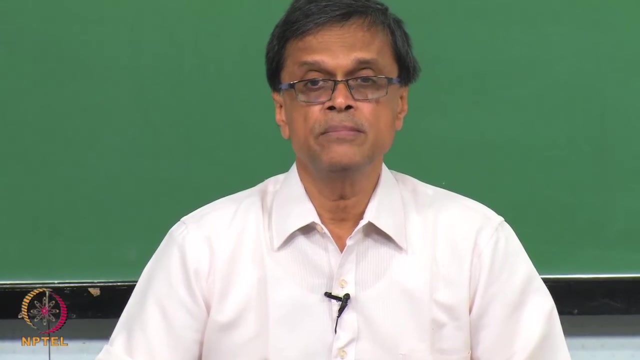 or coating antibacterial material. Yesterday I talked about coating heparin. When heparin is coated, it prevents the complement activation or even platelet activation, immobilizing enzymes and so on. There are so many different ways of modifying the surface so that we 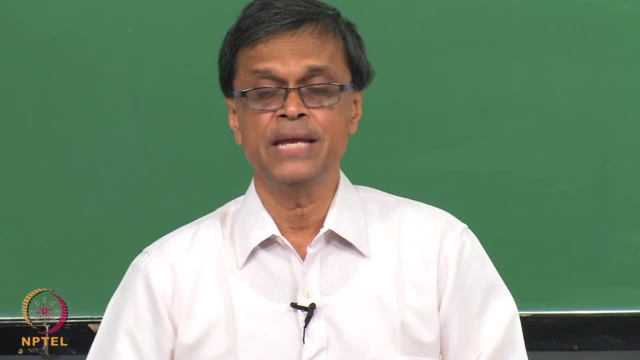 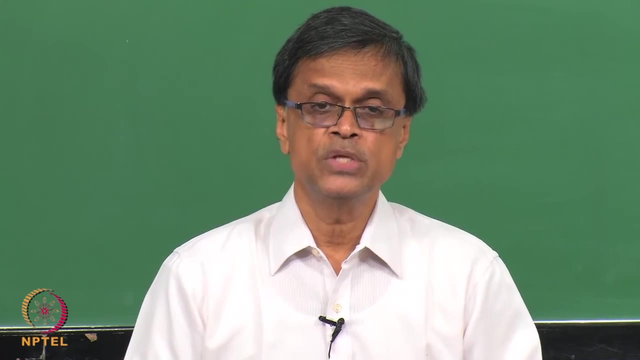 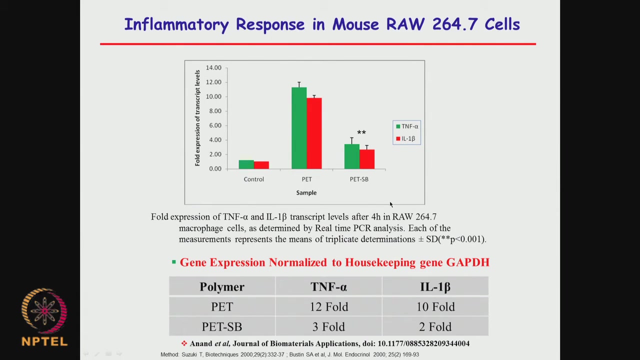 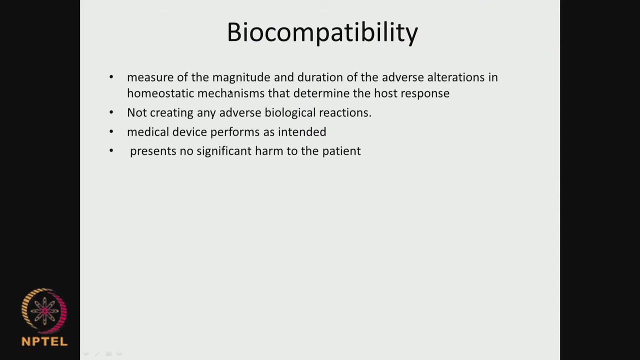 can reduce the blood coagulation, we can prevent the activation of platelets, we can reduce the inflammatory responses and so on actually. So this type of in vitro study is very, very important before you actually do it Go into in vivo animal studies. So biocompatibility, basically measure of the magnitude and duration. 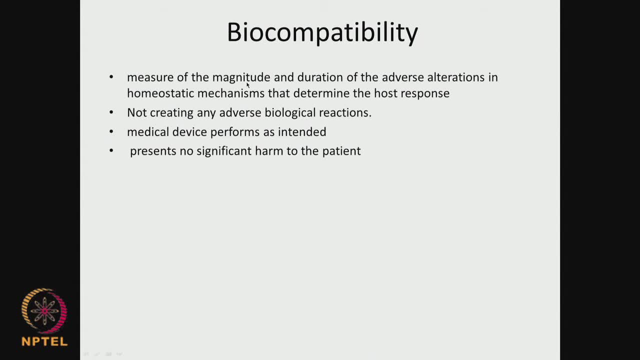 of the adverse alterations. It is not only how bad the response is, but how long it lasts in the hemostatic system in the host. It should not create any adverse biological reactions. At the same time, the medical device should perform as intended. 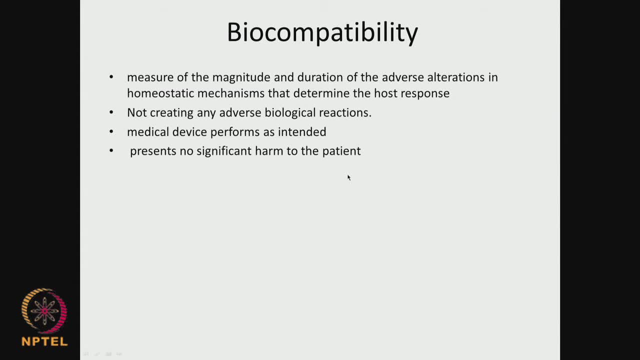 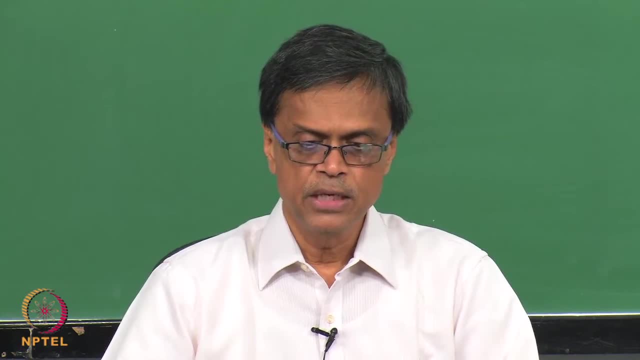 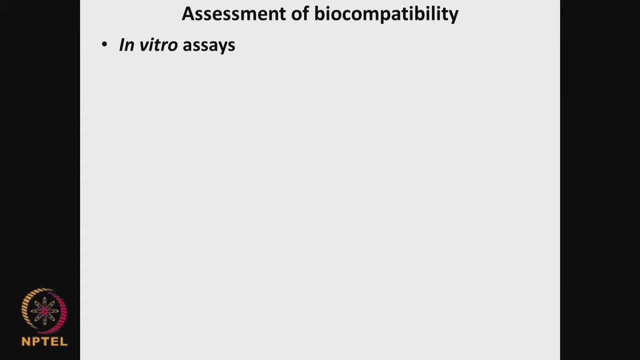 It should not present any significant harm to the patient. So these are all necessary. when you want to say the material is biocompatible, So many assays are there for assessing biocompatibility- I have been talking about it in previous classes also, So sort of. we will summarize them. There are in vitro assays. That means we 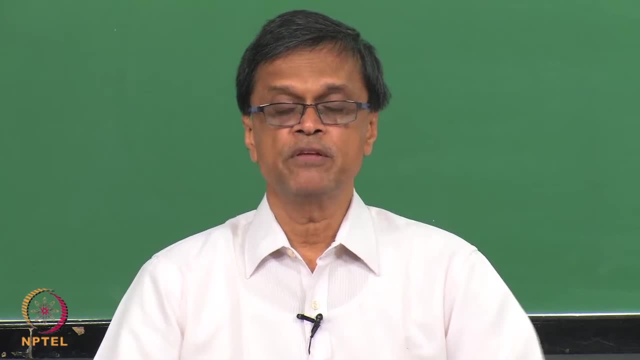 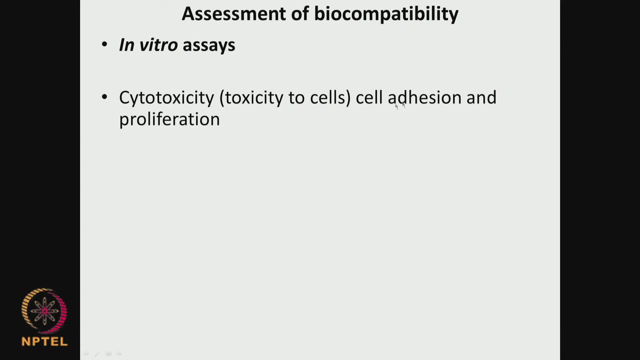 can do it in lab. There are in vivo assays where you do it in animals. So in vitro assays. I mentioned it long time back: cytotoxicity, Toxicity to cells, cell adhesion. that means, are the cells adhering properly and then are they proliferating properly? Is there a problem? 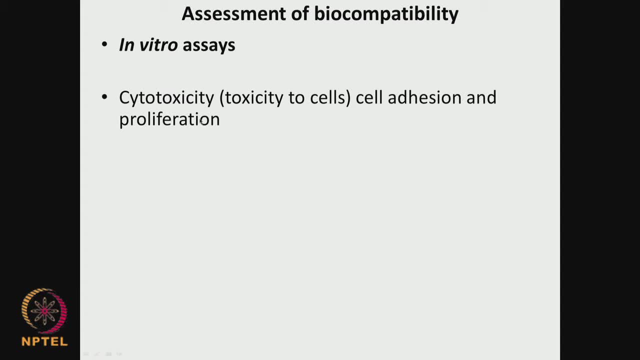 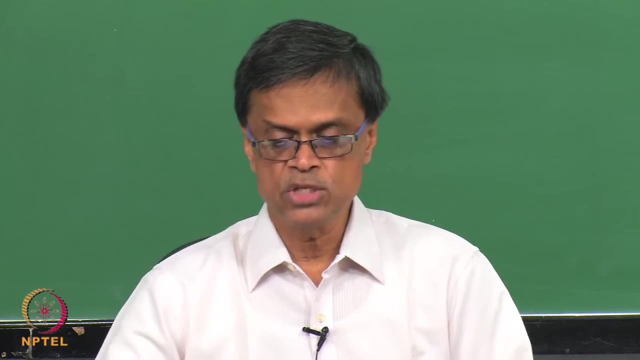 in adhering Is there a reduction in the proliferation. That means cells are dying, cells are not growing. That is called cytotoxicity. So we are looking at cell death, altered membrane permeability, So as the membrane become very porous, so some of the enzymes inside. 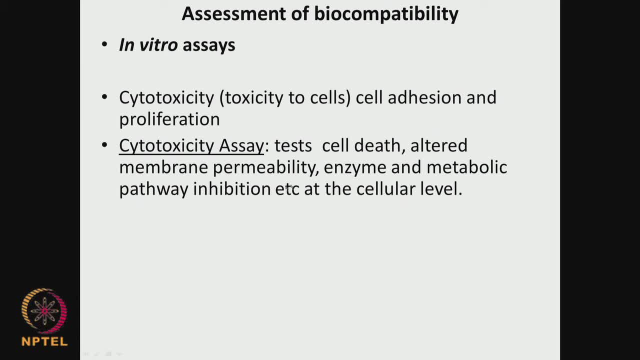 which are important, come out at the cellular level, So we can monitor even that also. We can look at whether membrane has become permeable using different types of dyes and looking under a microscope So we can have fluorescent dyes and if the membrane is permeable. 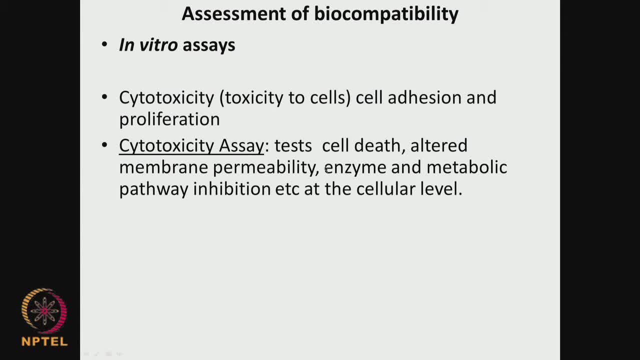 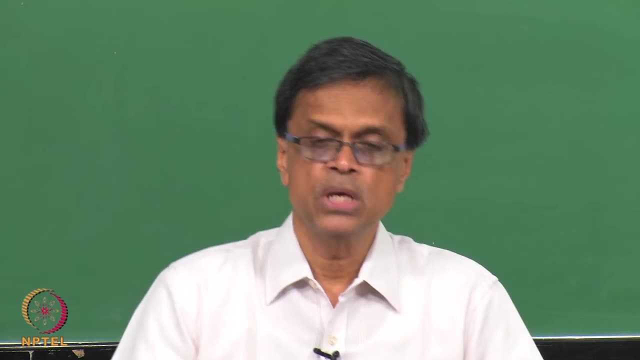 then those dyes may go inside and then we can look at it using a microscope, fluorescence microscope. We can also look at Specific cells. There are so many different types of cells we can look at. We can look at, like I showed you in the previous case, mouse cells. We can look at human L6 muscle. 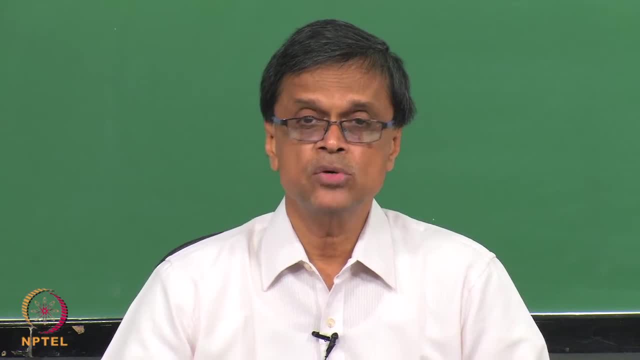 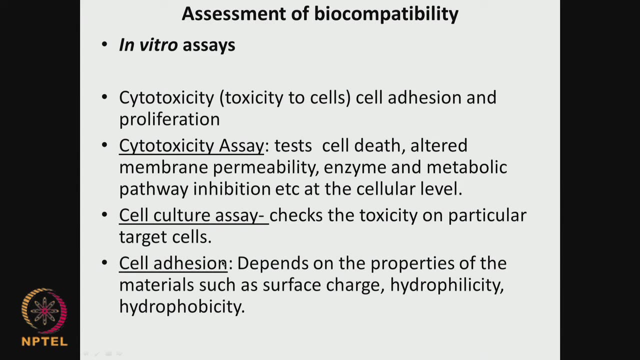 cells. We can look at bone marrow cells, so on. So we can look at the cell culture on specific cells. So then we can look at whether the cells are adhering properly, because that is also very important. Adhesion is very important so that the cells 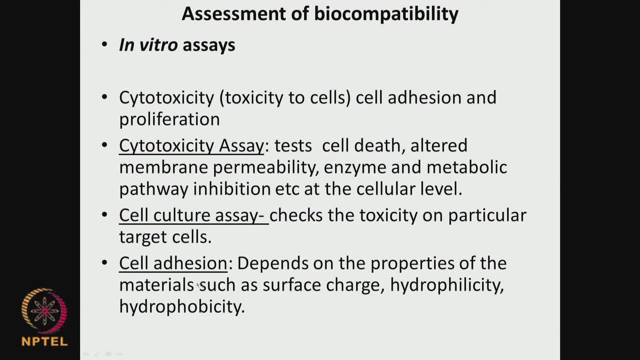 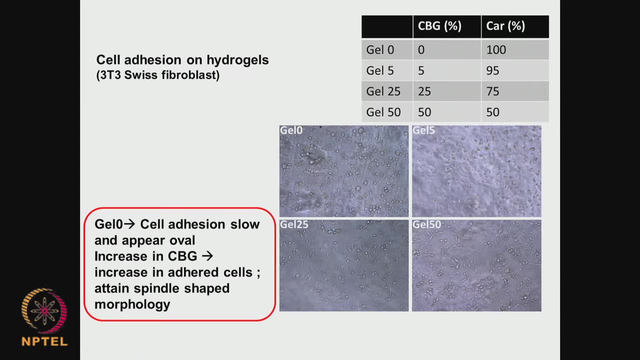 can start proliferating. So the adhesion depends on the properties of the biomaterial, like surface charge, hydrophilicity, hydrophobicity, what is the surface roughness, and so on. So we can do that sort of cell adhesion studies experimentally in the lab, in vitro based. 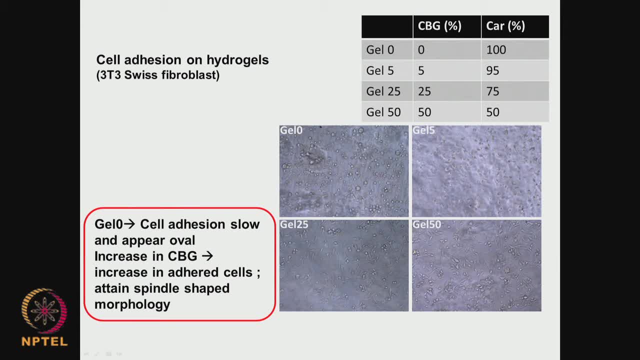 For example. I just want to show you an example of how to do. What we did was we have a biomaterial made where we use different types of beta glucon. Glucons are produced by bacteria. These are all bacterial glucons, So they are generally. some of them are water soluble. 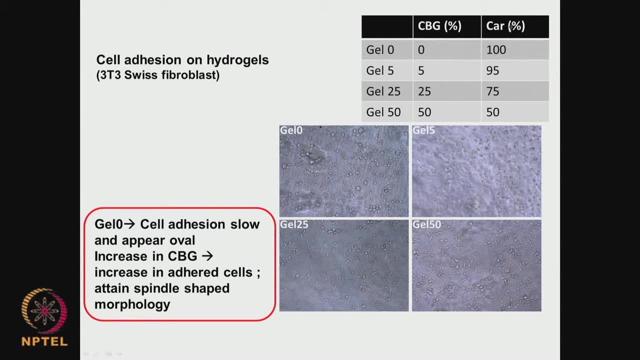 In this particular case, this is water soluble. They are very biocompatible. This is carrageenan. So we prepared 4 types of gels: One with the no glucon, only carrageenan. beta glucon, it is called. Beta glucons are also supposed to be immunomodulating properties, So beta. 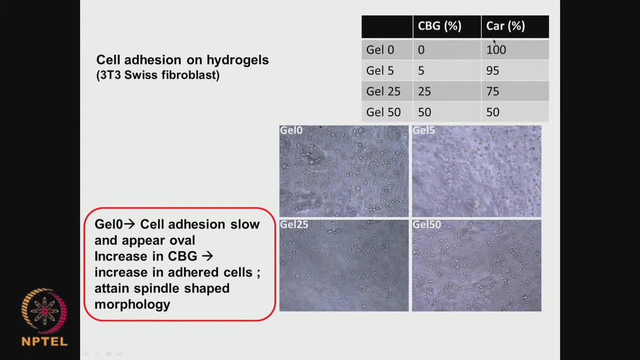 glucon and this gel is prepared only with 100% carrageenan. This gel is prepared with 5% beta glucon and 95% carrageenan. This gel 25 is prepared with 25% weight and 75% carrageenan. 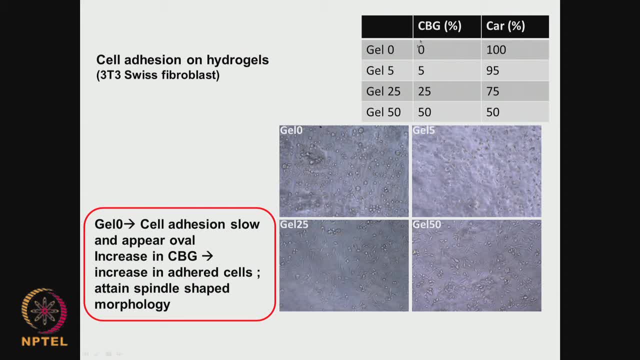 This gel is prepared 50-50.. So 4 different gels with increasing beta glucon. As I said, beta glucons are produced by bacteria. They are biocompatible. They are water soluble. Some of them are water soluble. In this particular case, it is water soluble Molecular weight. 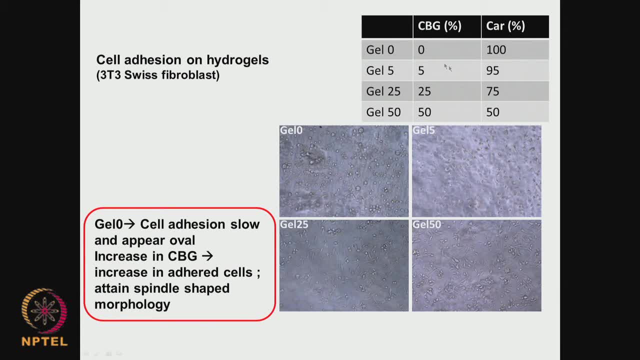 about 1500 daltons and then we grow cells on them. We grow this particular cell, 3T3, swiss fibroblast. So look at this: On gel 0, that means there is no beta glucon, only carrageenan. Cells are not adhering properly and the cells have to look spindle safe. So 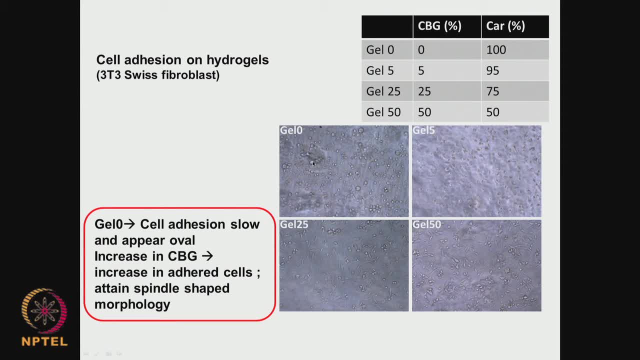 these are the cells. Cells look spindle shaped, whereas they all look spherical shaped. Obviously, this particular material surface is not very conducive, So it is toxic to the cells. 3T3 cells. Now look here: As we keep adding beta glucon- 5%, 25%, 50%- you can see cells are becoming spindle. 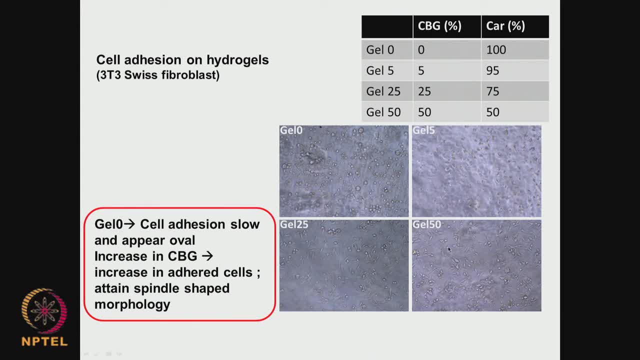 shaped. This is the correct morphology of the cells. They are becoming spindle shaped here. Very nice, very nice. So by adding more beta glucon, which is biocompatible, you are allowing the cells to adhere as well as grow in a proper shape, which is the spindle shape. 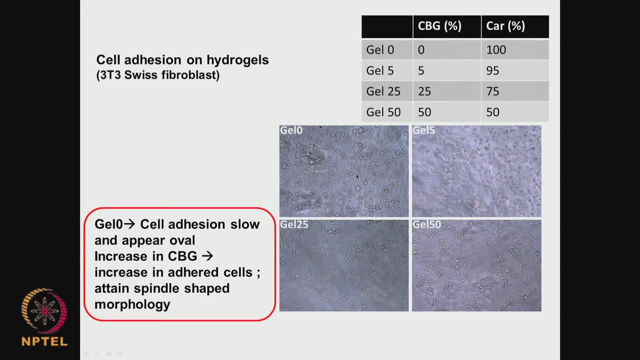 Whereas if you look here, when there is no beta glucon, they are spherical. Obviously this is not the correct. So addition of beta glucon is improving the biocompatibility of the material. So you can do this type of studies in vitro in the lab. So the amount: 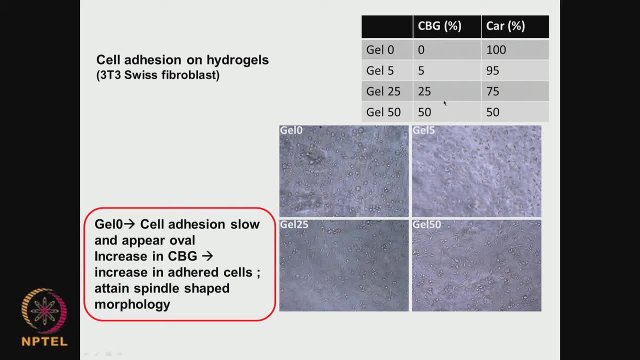 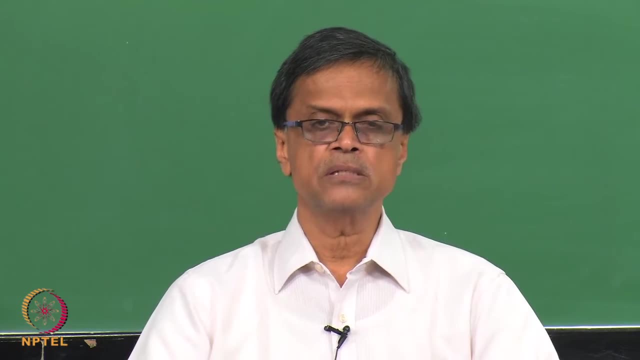 of adhered cells also increases As you increase the beta glucon and they also achieve their spindle shape morphology. You can see this. So these are called adherence tests, which are carried out in vitro. We can look at any type of cells and then we grow the cells and 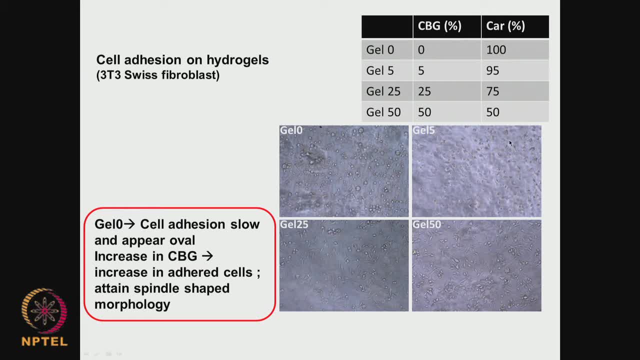 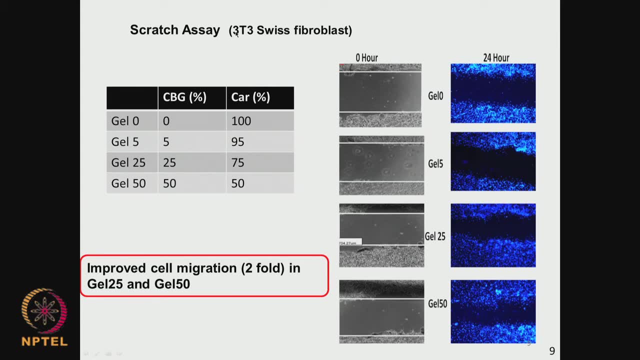 then we can look at them under a microscope. So it is quite easy actually. You can do another study that is called scratch assay. This is again an in vitro. In vitro means you can do it in the lab. The scratch assay tells you whether the cells are migrating. 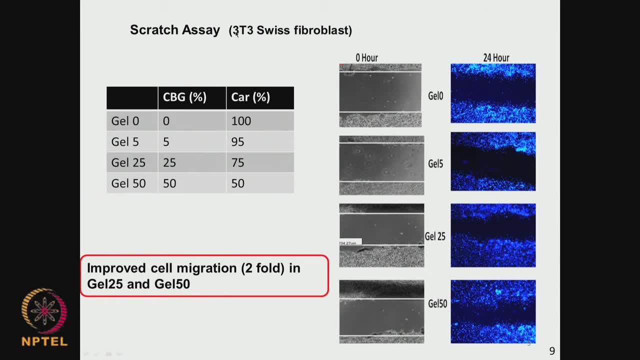 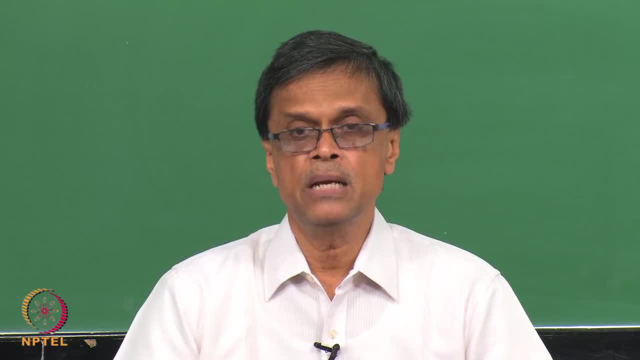 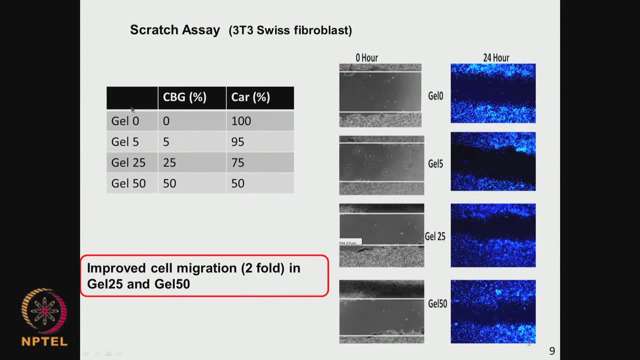 That means they grow and start migrating. If the surface is very biocompatible, cells will nicely migrate. The surface is not biocompatible, it is toxic. then the cell migration will be slow or completely retarded. Say same material. we took 4 different surfaces. This has got 100% carrageenan, This gel 5. 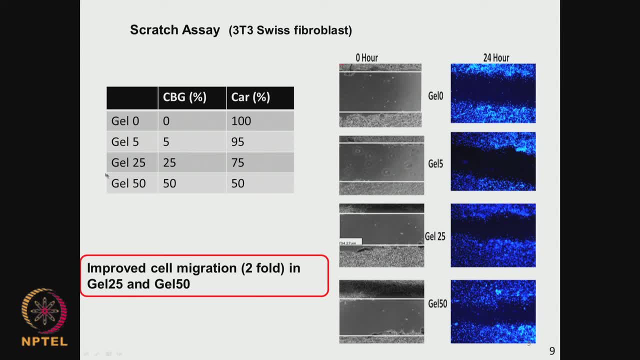 has got 5% beta glucon, 95% carrageenan. This gel 25 has 25% beta glucon, 75% carrageenan. This gel has 50-50 beta glucon and carrageenan. So what you do is we grow the cells, we 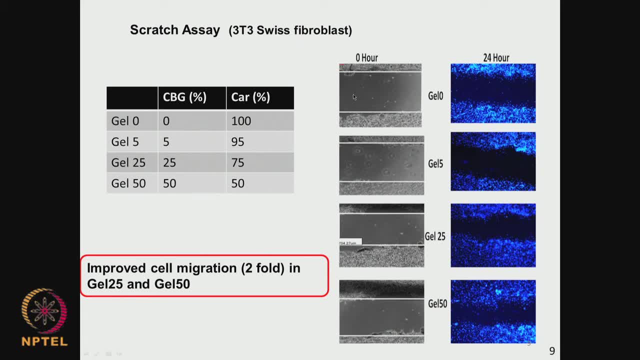 keep them alive for 24 hours and then we create artificially a scratch. Scratch means we make a mark with a very fine needle and then we start seeing whether the cells start migrating. So slowly, slowly, the scratch should completely disappear. So this is 0 time. This is 0 time. 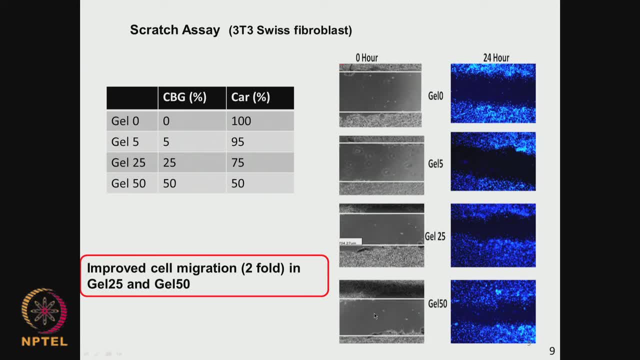 on gel 0,, gel 5,, gel 25,, gel 50. We created a scratch and then, after 24 hours, we are monitoring the scratch. This is a colour image. We have put in a dye So you can see only carrageenan. 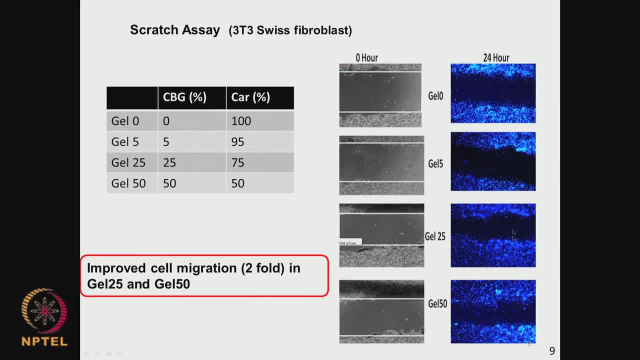 is there. The gap is very large, whereas the gel 50, which is 50-50, carrageenan beta glucon, the gap is very small. That means cell has proliferated, migrated and started reducing the scratch. That means the material is very conducive for the cell growth. It is a very 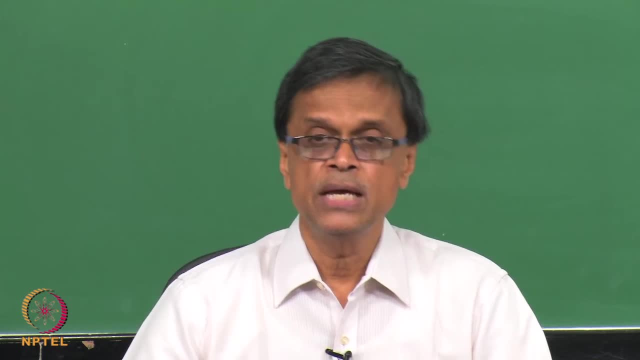 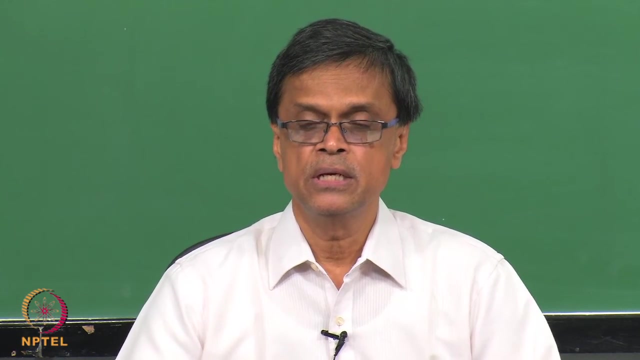 interesting experiment Which you can do in in vitro, and this experiment also tells you we can use this type of material because they help the cells to proliferate, migrate, which are very, very important if you want to have a very highly biocompatible biomaterial, Whereas this particular gel. 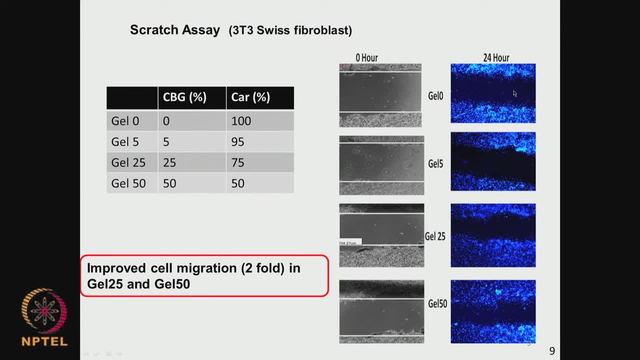 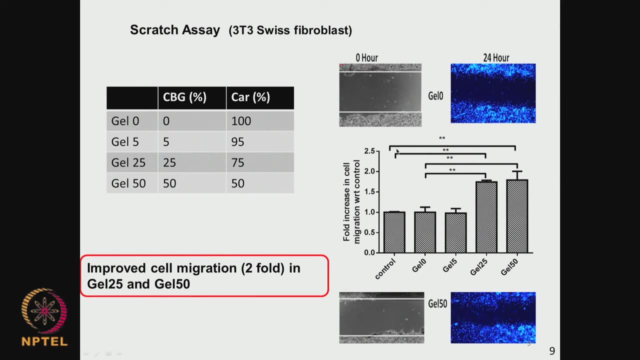 0, which is 100 percent carrageenan. look at this: Even after 24 hours, the migration is very poor. That means it is slightly toxic. As you keep increasing the beta glucon, you can see the migration. the proliferation is very, very good. This is shown numerically here. So 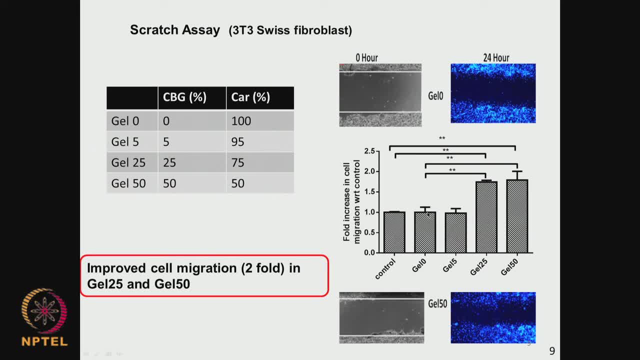 gel 0 migration. if you take it as 1,, the 25,, 50,, the migration goes to almost 2 times. So double the rate at which cells are migrating. When you increase the beta glucon, the migration こんo 1 times. It starts to increase because the migration is increasing. So the beta glucon is increasing. It goes 20 times. This is shown numerically here. So gel: 0 migration. If you take it as 1, then 25 and 50. the migration goes to almost 2 times. So double the rate. 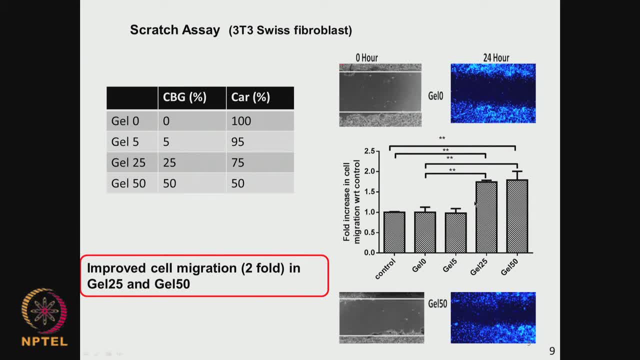 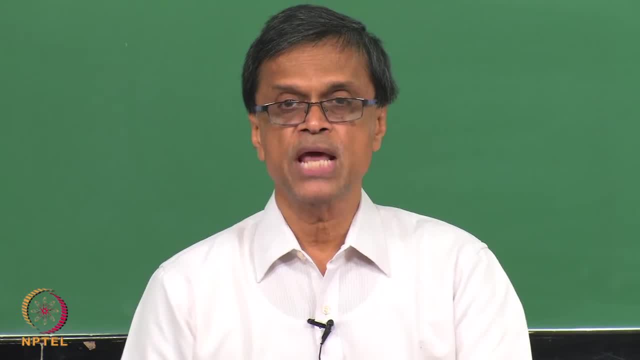 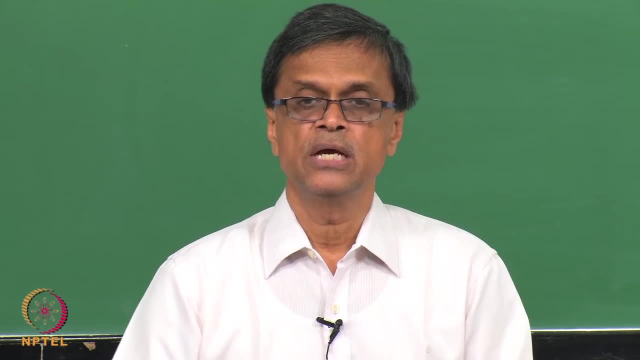 So these assays, the in vitro assays I talked about in the previous slide, the adhesion and the morphology development and the scratch assay- all these assays are very useful to determine whether a biomaterial is conducive to cells. These are experiments done in vitro, that means in the lab. 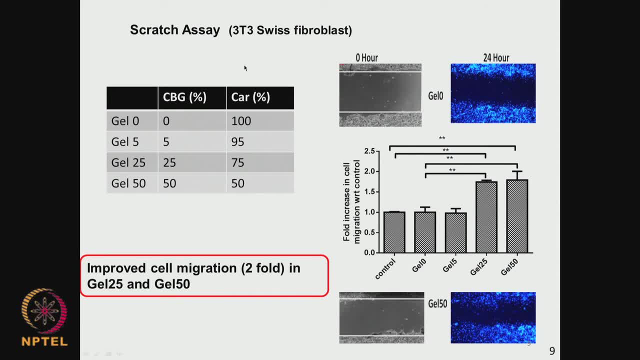 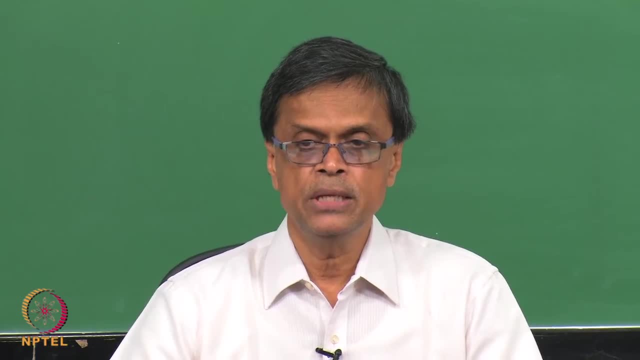 So we can use different types of cells. as I said, you know, here I am showing you 3T3, we can use raw cells, mouse and so on actually. So I showed you lot of different in vitro based experiments monitoring the inflammatory. 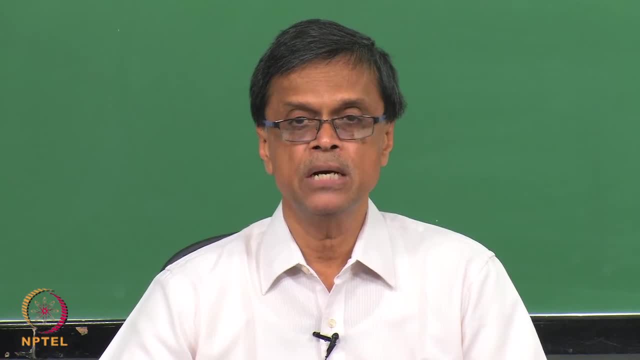 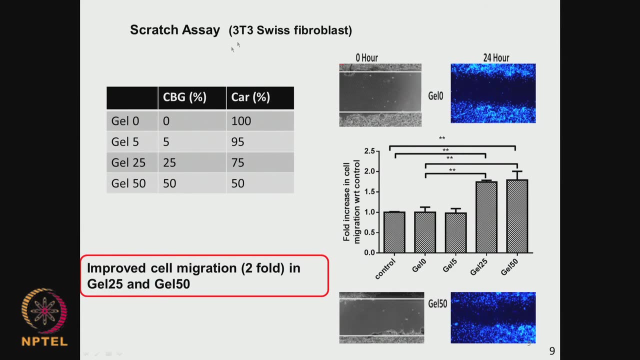 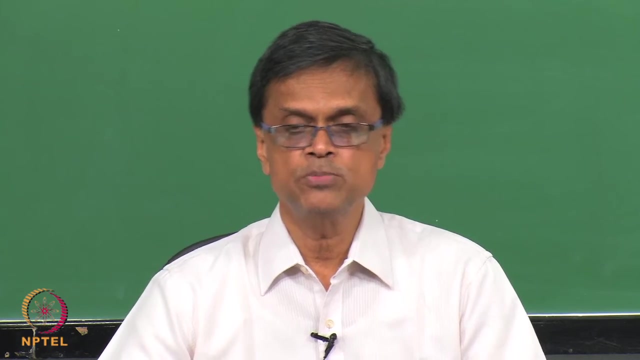 markers like TNF alpha or IL-1 beta. looking at cell adhesion proliferation, looking at the cell migration using this scratch assay. all these are experiments which we carry out in the lab. 2. We can prove or disprove whether a material is compatible or non-cytotoxic. 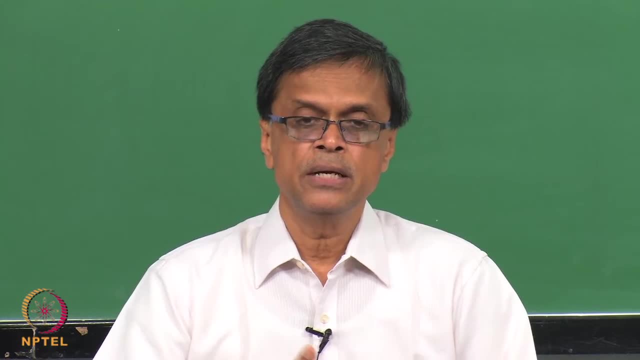 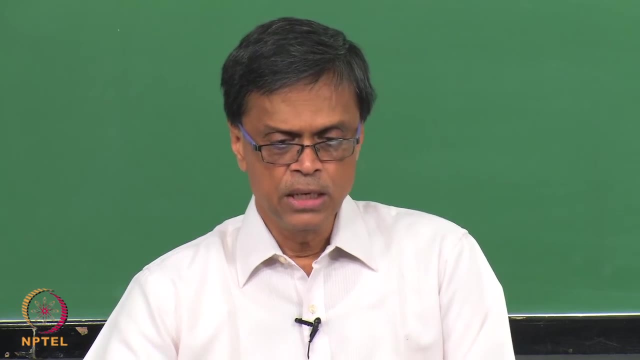 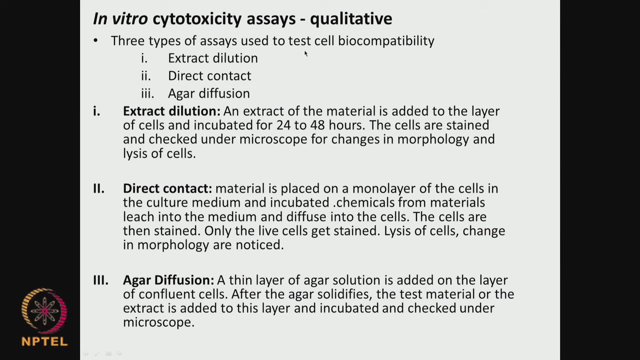 Then we can modify the surface and again see whether the cytotoxicity is reduced. Finally, once we are satisfied, we can go to animal studies. So the in vitro cytotoxicity assays is: we take the material polymer, for example. we 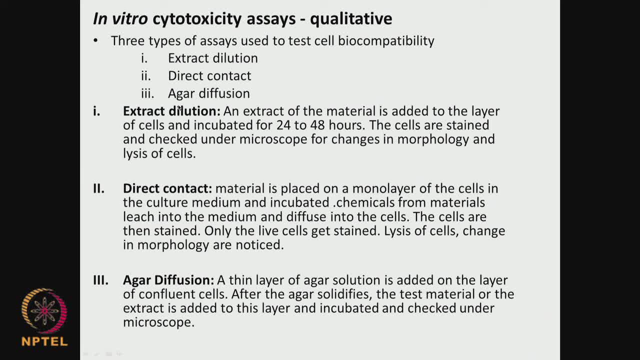 see whether the extracts from the polymer 3.. The extracts from the polymer are going to create toxicity. this is very useful, especially in dental implants. For example, dental PMMA polymethyl methacrylate is used widely. how do they do they take? 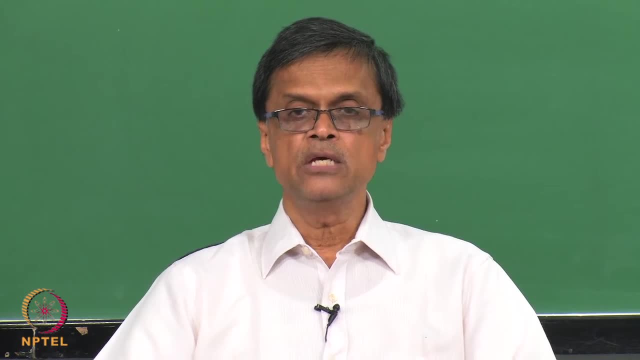 methacrylic acid and it is polymerized using UV. so most of the methacrylic acid is becoming polymer. most methyl methacrylic acid becomes polymeric methyl methacrylate, but little bit of monomer is left behind, little bit. 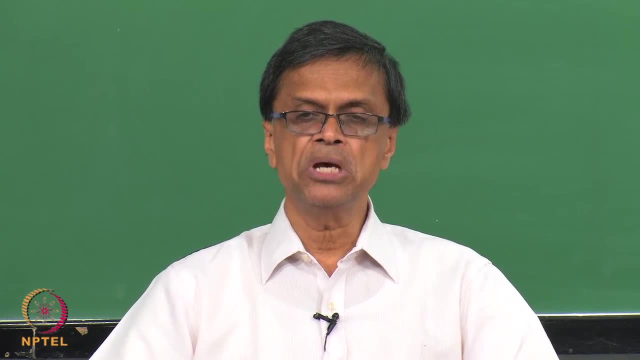 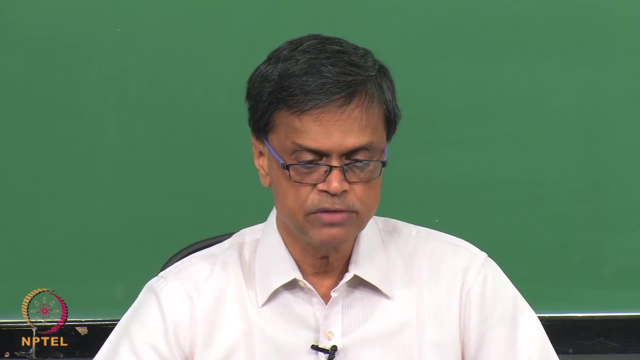 4.. So this is a type of assay which may slowly leach out over a period of very, very long time. So is this leachance toxic? so this type of assay is very useful. So what we do is we extract from the polymer and use that extracted solution and see whether 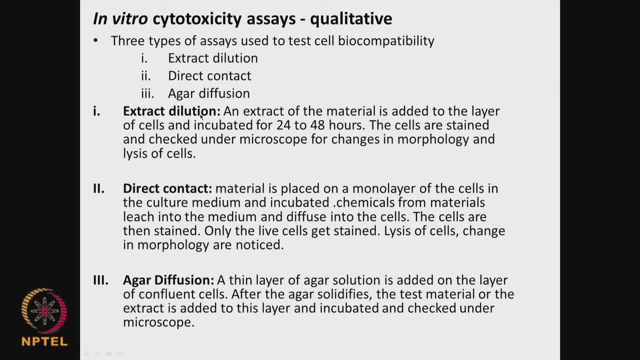 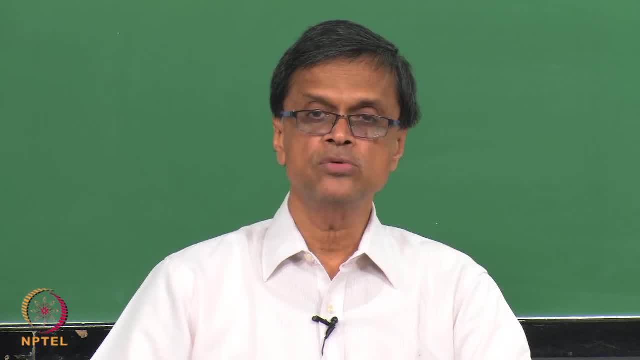 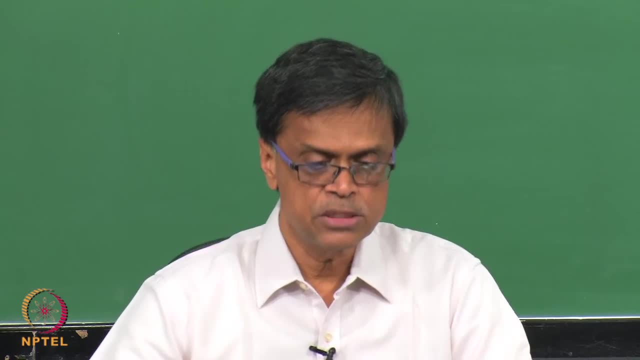 the cells grow in that, whether the cells die in that and so on. actually, For example, you are using amalgam. lot of amalgam based materials are used in dental fillings, So they can slowly leach out over a period of years. so are they toxic? 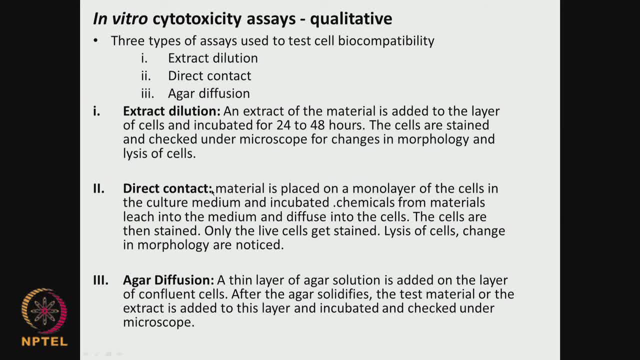 So this particular assay is very useful. so you take out the samples, extracted liquid from the material and then test whether that liquid is toxic to the cells. 5. Direct contact. so what do you do? you incubate the material, biomaterial, with the cell lines. 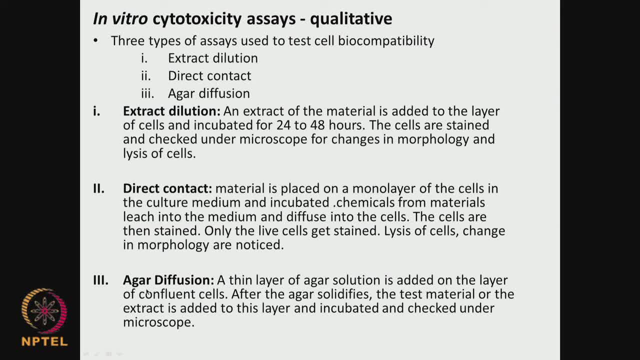 and that is called direct contact. Third approach is called agar diffusion 6. So what you do is: we have cells nicely growing, so we add a thin layer of agar solution on top. Agar is used for growth of cells, bacteria and so on. 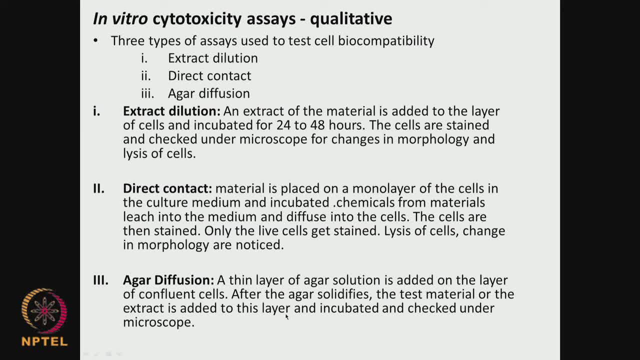 Then, once the agar solidifies, your biomaterial is added to this and then you check. so if the biomaterial is toxic, the cells will not grow closer to the biomaterial, but if the biomaterial is not toxic, Cells will completely grow even near the biomaterial and start engulfing it practically. 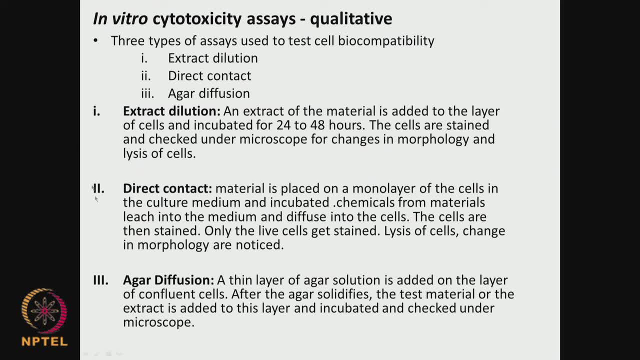 That is called the agar diffusion. So this method is almost like your cell attachment and proliferation and migration, whereas these two methods are like cell proliferation or cell death 7. So these are in vitro methods. These are more qualitative Because we cannot get a quantification. 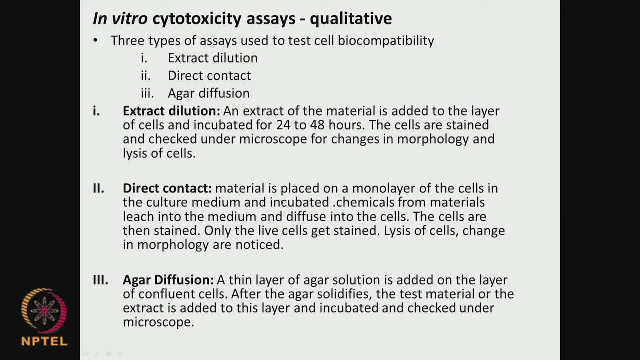 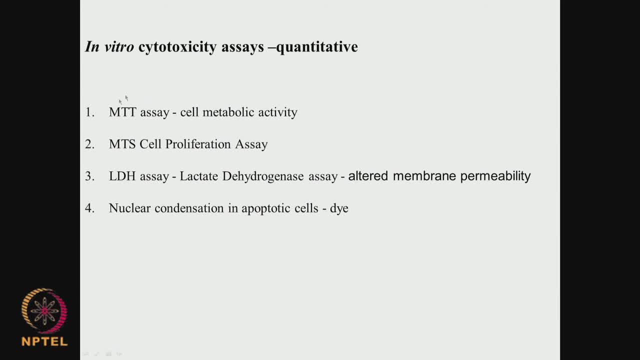 8. So we cannot get a quantitative number, but there are quantitative methods are also there. I talked about it long time back. If you remember, we used to do MTTSA. do you remember? In our old class we did. otherwise, you can go back and check. 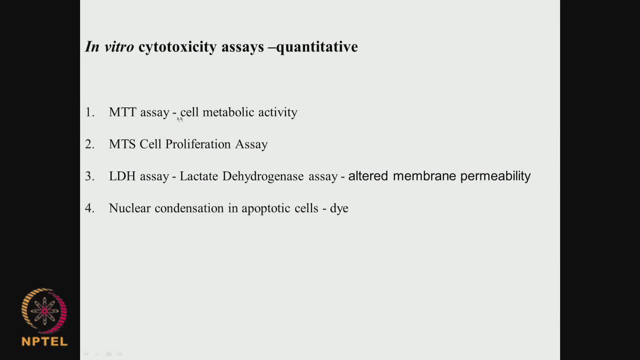 It tells you the cell metabolic activity so we can calculate in percentage. with respect to control how many cells are viable cells are there. We can say 90 percent viable cells, 80 percent viable cells, Something called MTSSA. it is again looking at a cell proliferation, percentage of cells. 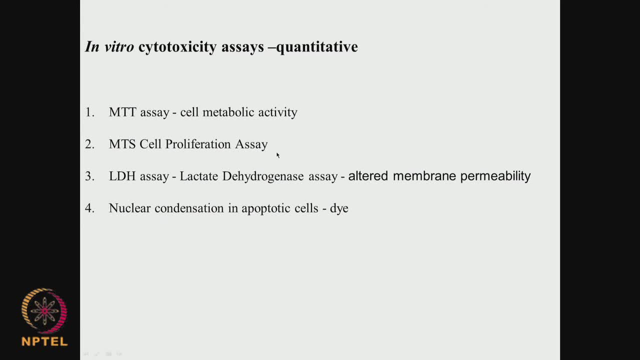 alive when it is with the biomaterial. with respect to the control. where we do not have a biomaterial, Then we have the LDHSA, because there is this particular enzyme called lactate dehydrogenase which is present inside the active cells or cells which have a good metabolic activity. 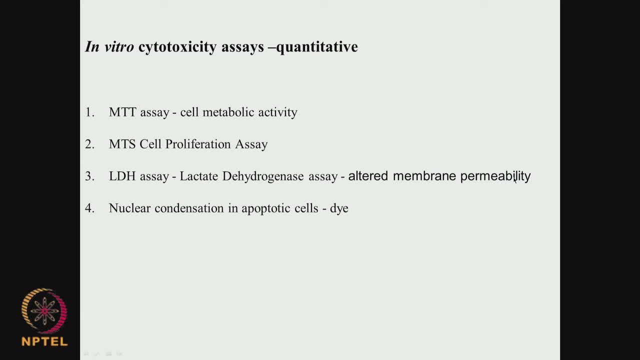 If the cells die because of necrosis, then the membrane becomes damaged. because of the reduction in membrane permeability, this particular enzyme comes out into the solution and the measure of the amount of this is a measure of the cell that has died because of necrosis or membrane damage. 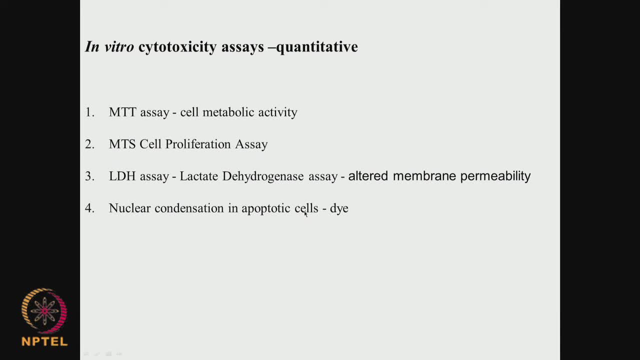 9. Another is nuclear condensation in apoptotic cells. So if the cells die naturally, which is called apoptotic, and we add some dye, we can see the nuclear condensation under a fluorescent microscope and we can tell whether it has died because of apoptotic. 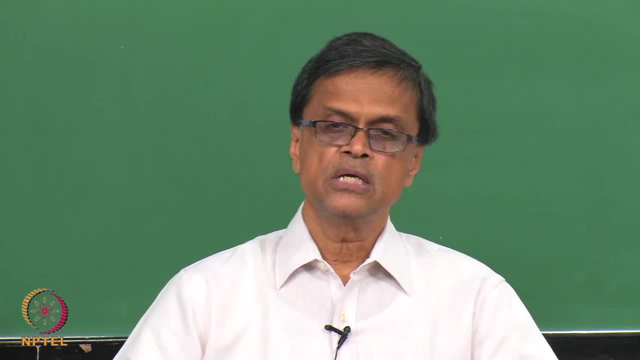 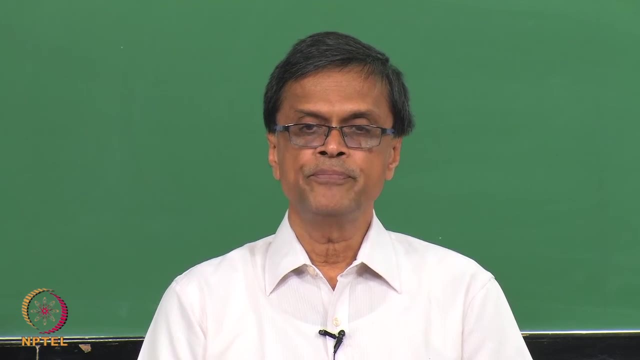 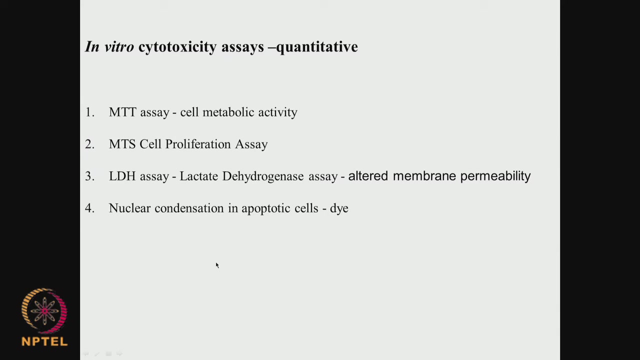 If it has died because of unnatural causes like necrosis, there would not be condensation of the nucleus. the nucleus will be spread all over the place, And so we can tell 10.. Next we have the necrosis. These are called quantitative assays- I talked about it sometime back- and these are the qualitative. 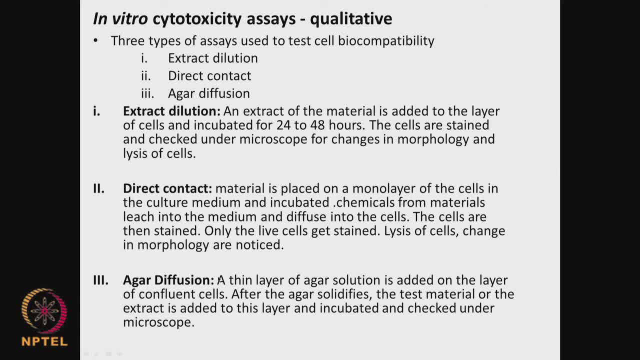 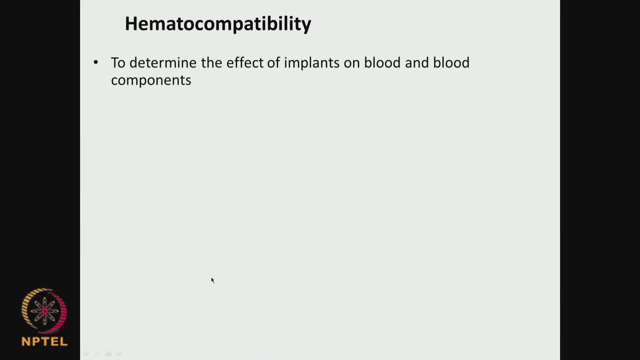 assays. So all these assays are very useful in vitro to understand the cytotoxicity. Then hemocompatibility, that is, the blood related compatibility. You want to know whether the effect of implant on blood and blood components. again, I talked about it long time back. 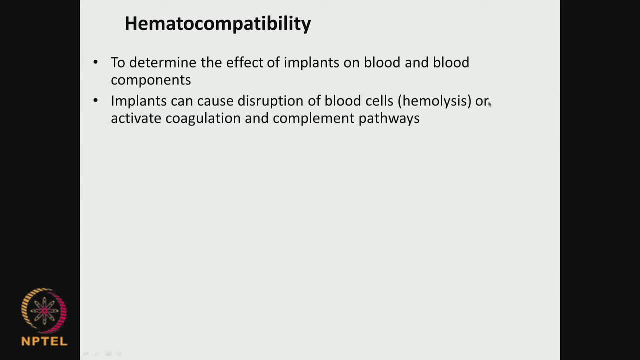 Because the implants can cause disruption of blood cells- that is called hemolysis- or they can activate the coagulation pathway leading to blood clots 11.. If you remember, we talked about fibrin and then complement pathway. So the implants can activate the complement pathway, which leads to several proteins getting 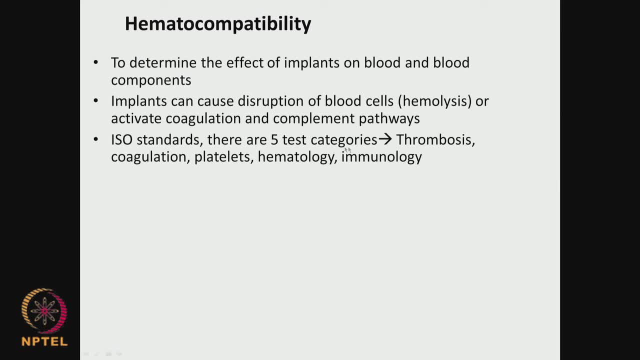 activated 12.. So the ISO standards are there, which talks about 5 different test categories: thrombosis, coagulation, platelet hematology, immunology. So one can do all these tests to understand whether the material is biocompatible. 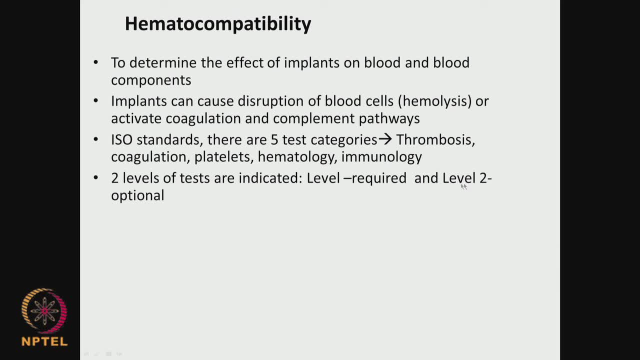 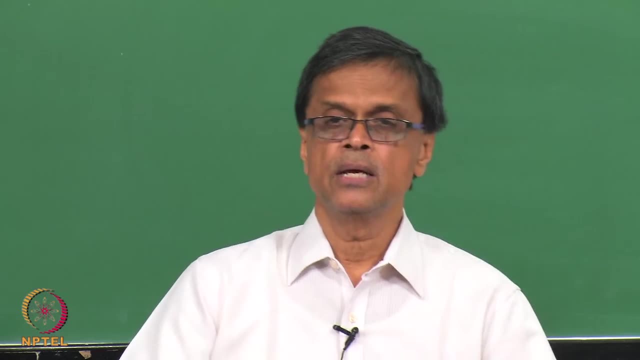 And there are 2 levels of test, the basic level and the advanced level. So again, the hemo compatibility depends on the material characteristics, fluid mechanics of the implant device, coagulability of the blood. So if somebody is having cardiovascular problem and he or she is given a blood thinning like 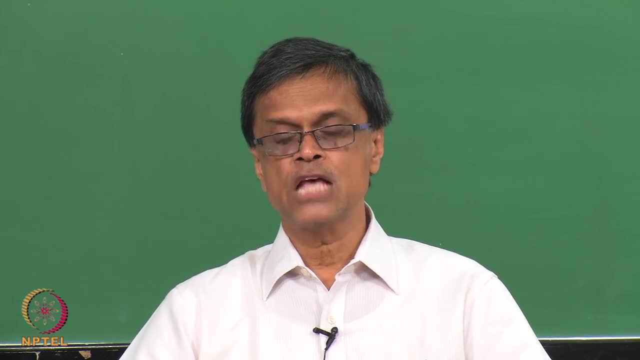 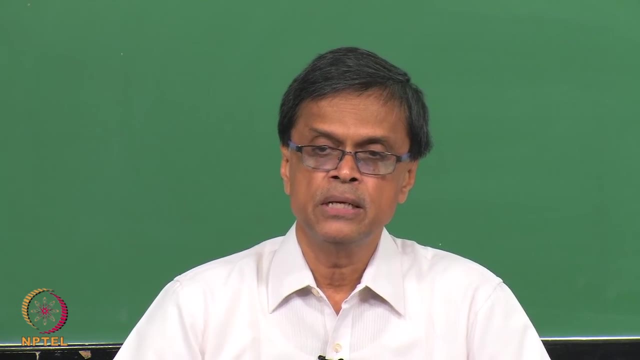 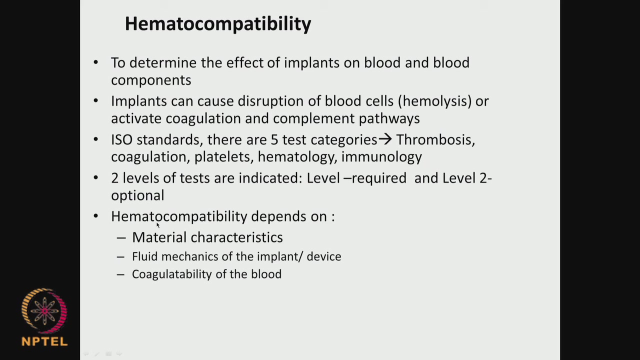 warfarin or even aspirin. So the coagulation does not happen so easily, whereas a normal person where the coagulation may happen easily. So hemo compatibility also depends on that 13. I also talked about how to reduce the activation of the coagulation, as well as the complement. 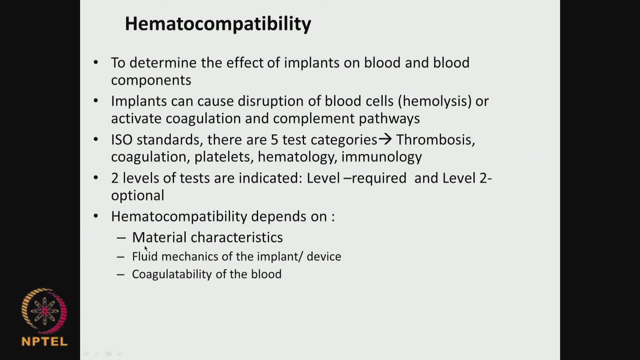 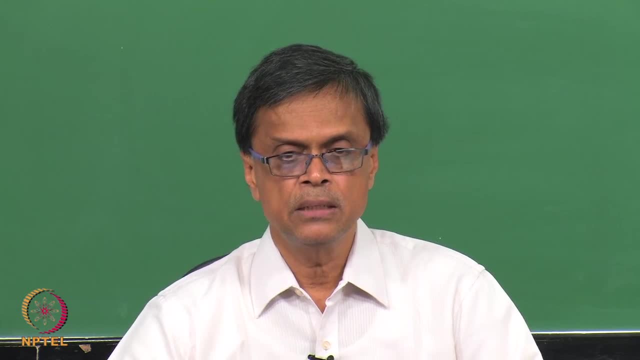 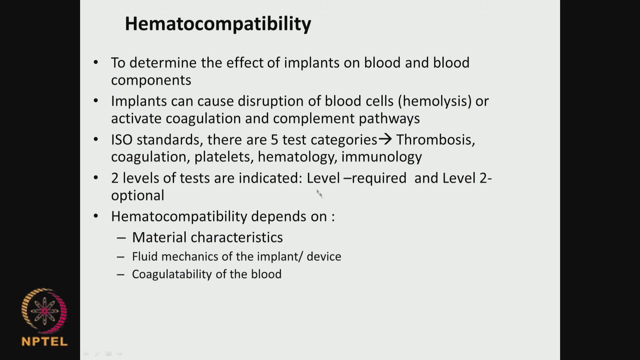 pathways, 14. There are coatings which can reduce that. we talked about it sometime back and we also said there are certain synthetic polymers which are very hemo compatible, 15., 16. And which does not activate these coagulation and complement pathways. 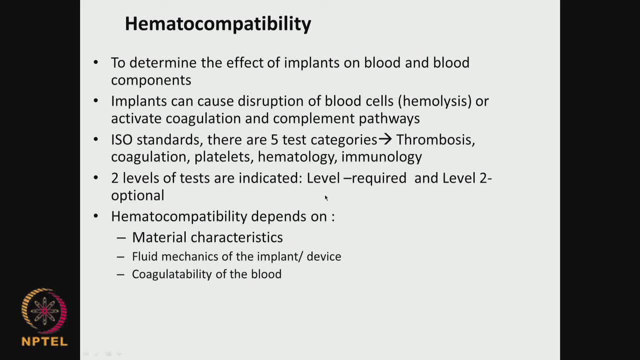 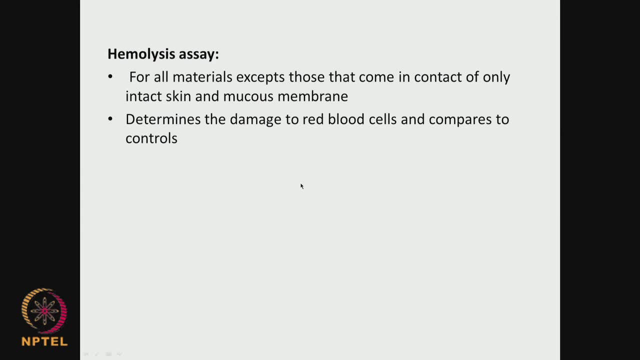 So one can think about using those biomaterials or think about coating the biomaterial which will reduce the activation of these particular 2 pathways. that is called hemo compatibility. So there is a hemolysis assay 17.. This is a hemolysis assay. 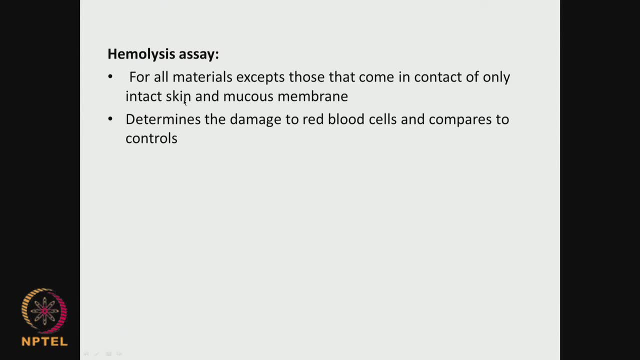 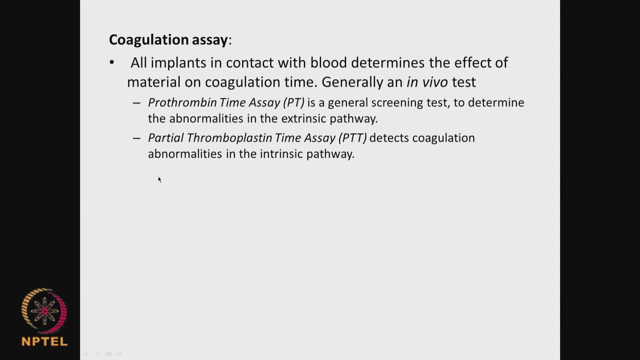 For all materials except those that come in contact of only intact skin and mucous membrane. So this assay tells you how much of the red blood cells are damaged with respect to the control 18.. So you also have the coagulation assay. 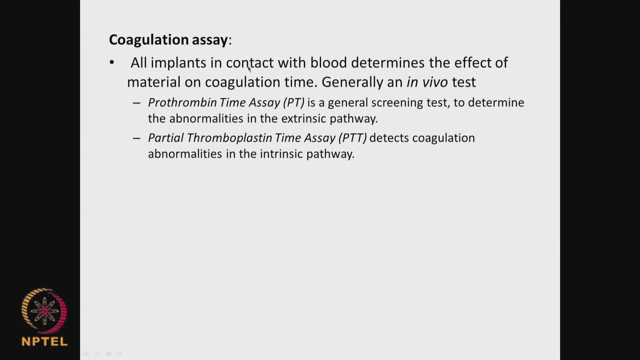 So it tells you the effect of the material on the coagulation time. One is called the prothrombin time, assay 19.. Other is called the partial thromboplastin time, assay 20.. Both these assays are quantitative. 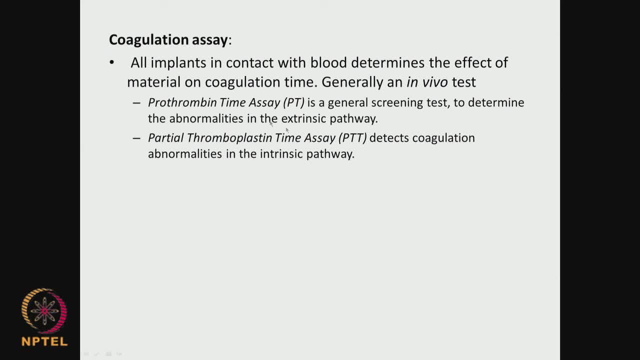 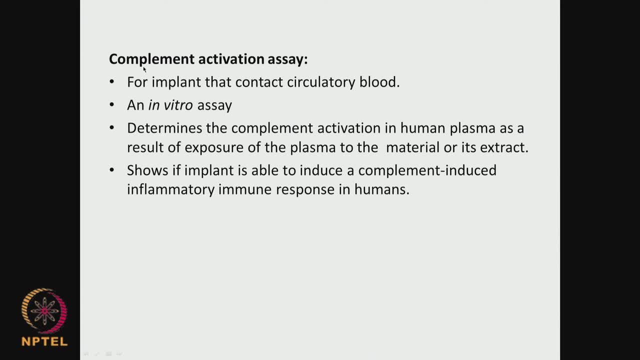 So it tells you the effect of the biomaterial on the coagulation with respect to the control. Control means without the biomaterial, 21.. Then there is argaine, assays for complement activation. So again, as I said, the complement activation with respect to the circulatory blood. 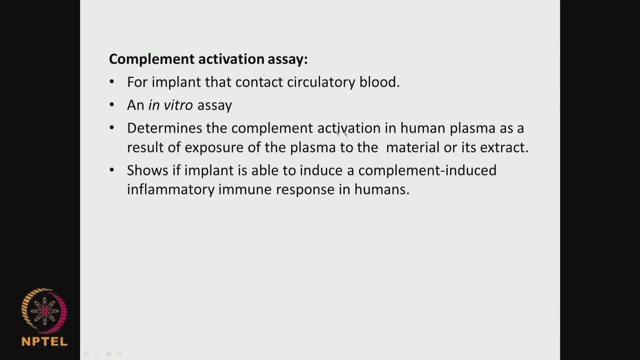 This is also an in vitro assay. So it determines the coagulation, It determines the complement activation in human plasma as a result of exposure of the plasma to the material. So this assay is very useful. It tells you whether the complements will get activated. 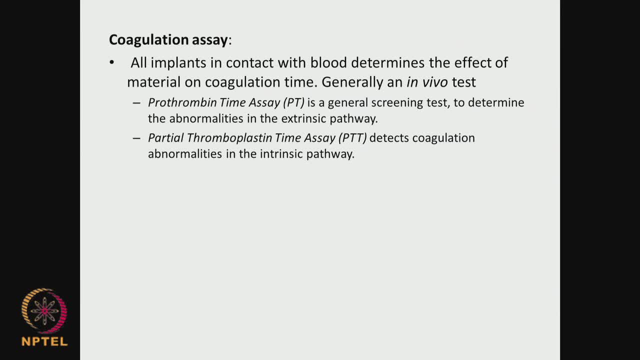 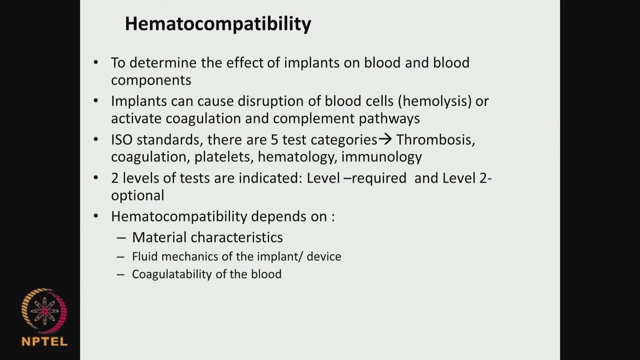 So we have the previous coagulation based assay or hemolysis based assay, which tells you whether the blood in the plasma getting going to get damaged, Whether the blood is going to get damaged, Whether the blood is going to get damaged 21.. 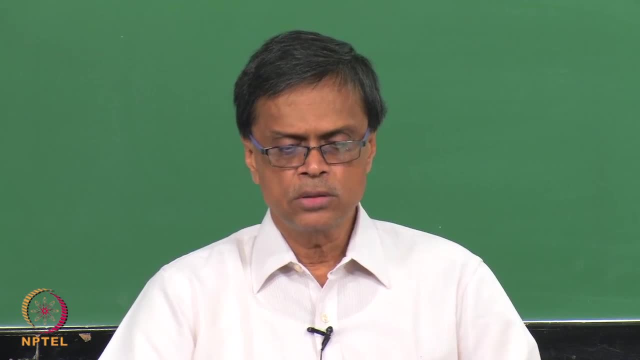 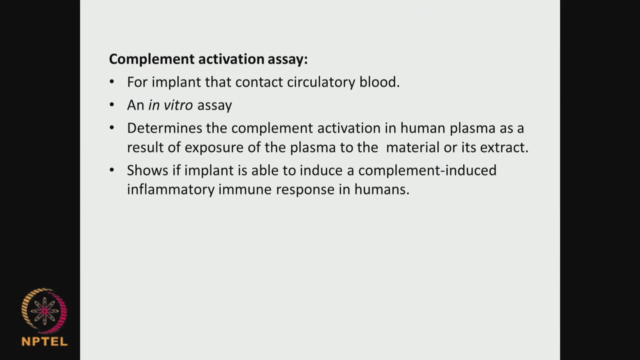 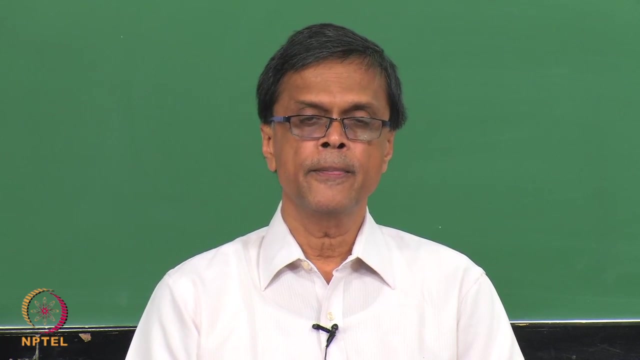 Then comes whether the biomaterial is going to activate your thrombosis and the coagulation pathway, And then comes whether the biomaterial is going to activate your complement system. So all these are assays, which tells you, sometimes qualitative, sometimes quantitative, the effect. 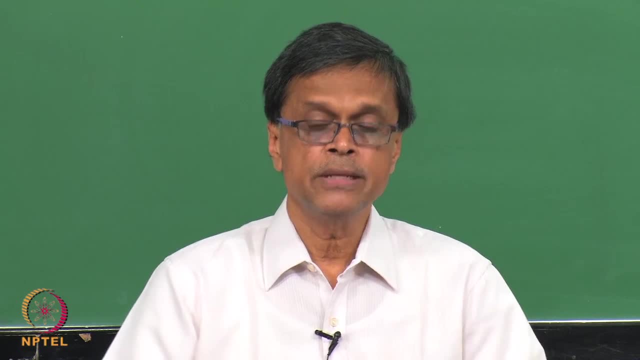 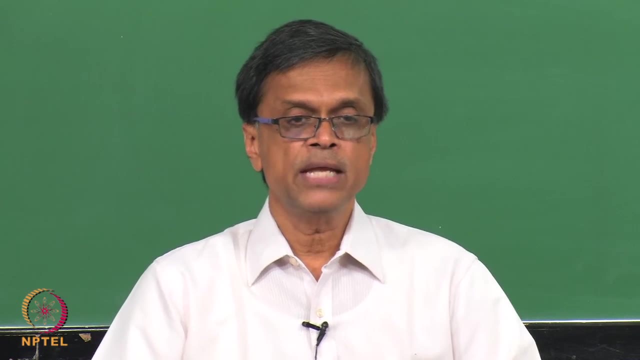 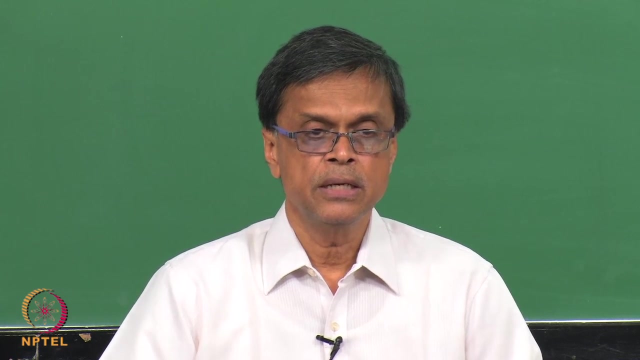 of the biomaterial. 22. On When: When they are coming in contact. So these are in vitro assays, So I can do it with cell lines, I can look at the gene expressions, I can take plasma, blood plasma, and then I can do experiments with the blood plasma and